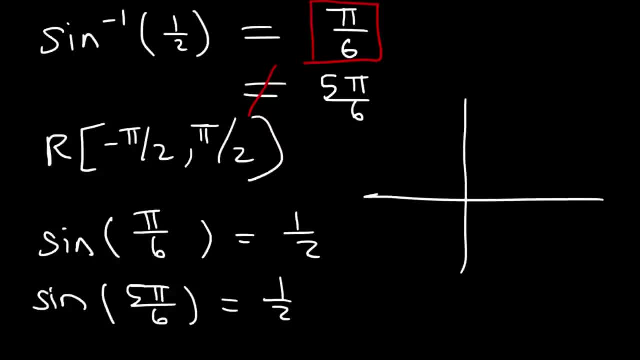 That is the answer. So, going back to the unit circle, you need to know that the arc sine function exists in quadrants 1 and 4.. So if this value is positive, it's going to be in quadrants 1 and 4.. 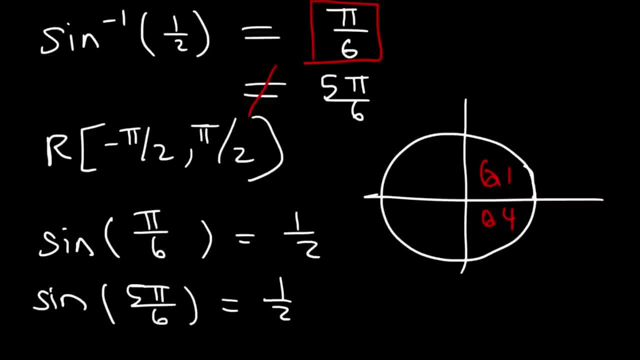 Because sine is positive in quadrant 1.. If we had a negative value, we need to use the answer in quadrant 4.. And we have to pick an answer that's within the range from negative pi over 2 to pi over 2.. 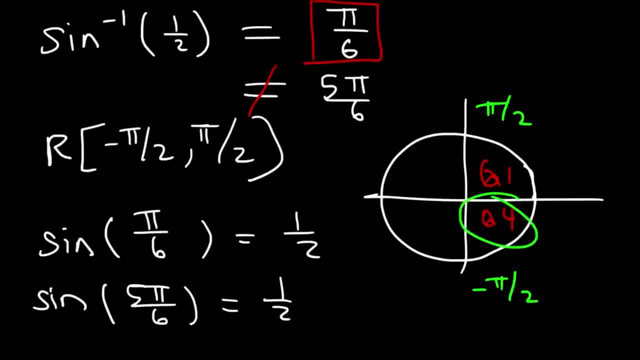 So even though quadrant 4 is between 270 and 360, that is not in this range- You need to use negative 90 to 90. So keep that in mind. Also, you can confirm this with your calculator If you type arc sine of 1 half. 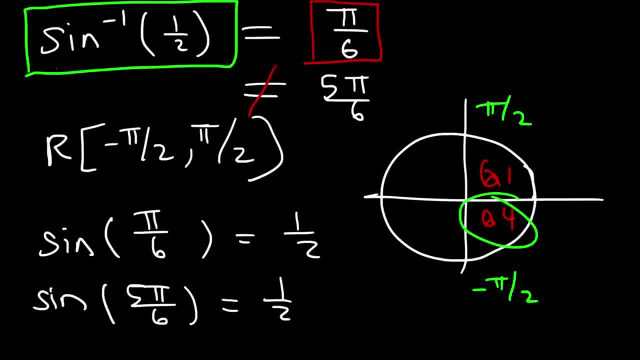 and if it's in degrees, you should get 30 degrees. You won't get 150, which is 5 pi over 6.. If you put in radians, then you should get pi over 6. Or maybe the decimal form of pi over 6.. 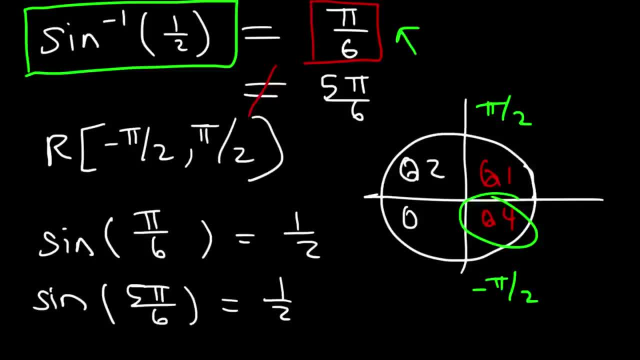 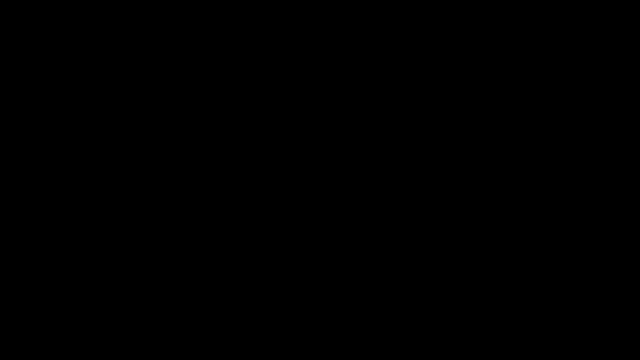 So arc sine does not exist in quadrants 2 and 3.. If you have an answer in these quadrants, you will get it wrong. Now let's work on some other examples. What is arc sine of the square root of 3 over 2?? 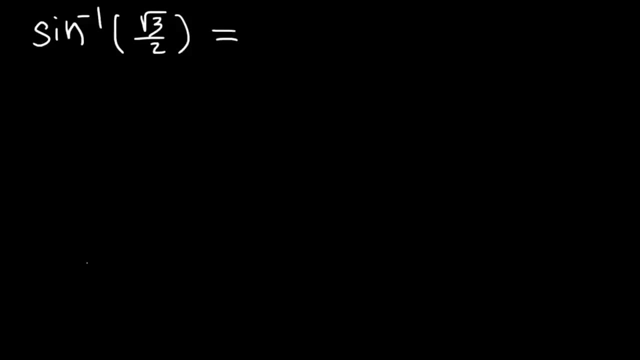 So go ahead and find the answer. Now we know that sine of- let's use degrees- Sine of 60 degrees- is equal to the square root of 3 over 2.. Also, sine of 300 is also root 3 over 2.. 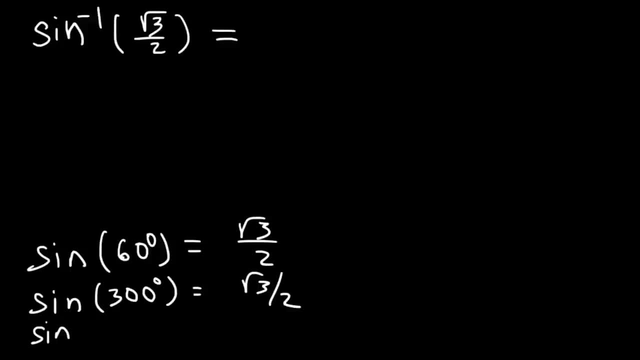 And at the same time I take that back. Sine of 300 is negative square root: 3 over 2.. Sine of 120 is positive root 3 over 2.. So we have two possible answers: 60 and 120.. 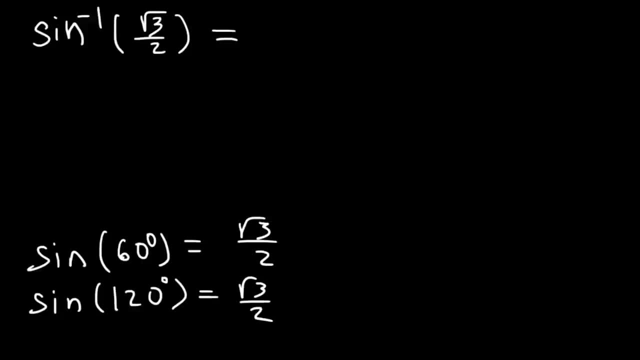 So which one should we use? Now? 60 is in quadrant 1,, which is okay. 120 is in quadrant 2.. And the arc sine function does not exist in quadrant 2.. So the answer is 60.. So the answer is 60.. 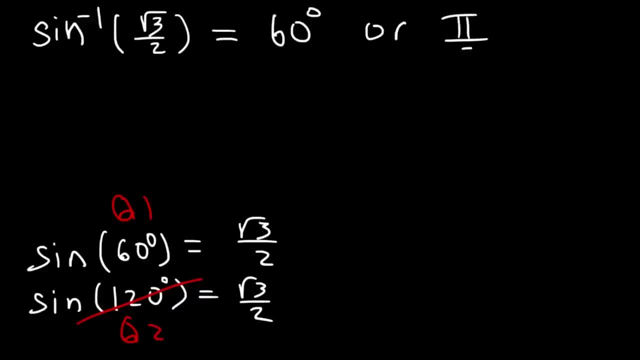 So the answer is 60 degrees, which we can write as pi over 3.. Keep in mind, pi is 180.. 180 divided by 3 is 60.. So that's the answer for this example. Arc sine of root, 3 over 2 is 60.. 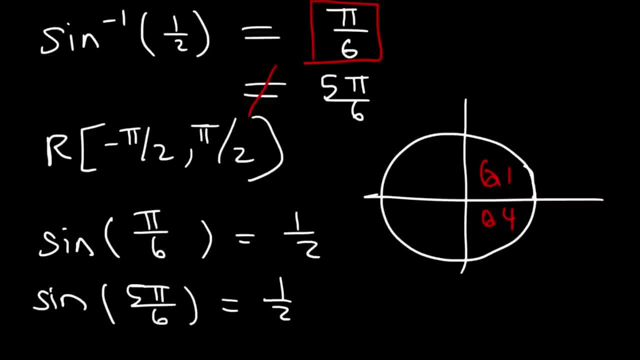 Because sine is positive in quadrant 1.. If we had a negative value, we need to use the answer in quadrant 4.. And we have to pick an answer that's within the range from negative pi over 2 to pi over 2.. 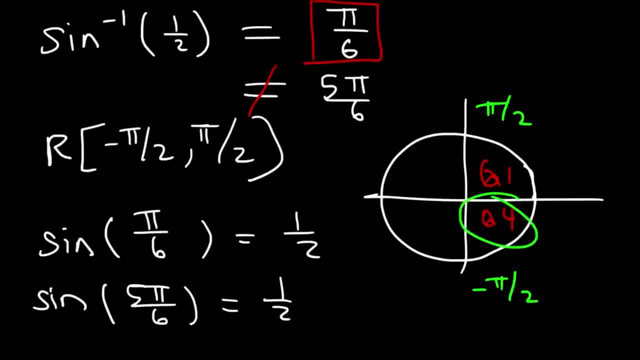 So even though quadrant 4 is between 270 and 360, that is not in this range- You need to use negative 90 to 90. So keep that in mind. Also, you can confirm this with your calculator If you type arc sine of 1 half. 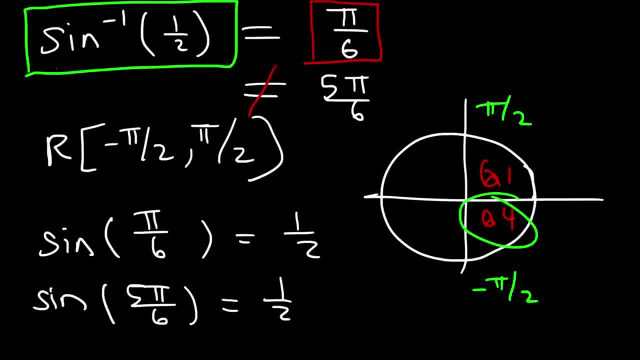 and if it's in degrees, you should get 30 degrees. You won't get 150, which is 5 pi over 6.. If you put in radians, then you should get pi over 6. Or maybe the decimal form of pi over 6.. 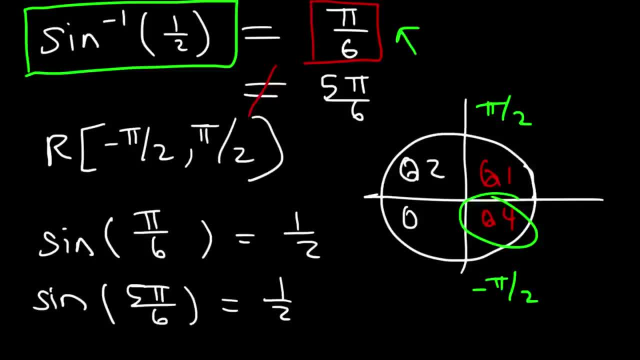 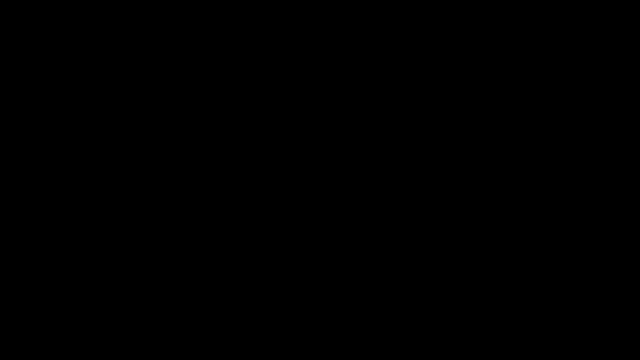 So arc sine does not exist in quadrants 2 and 3.. If you have an answer in these quadrants, you will get it wrong. Now let's work on some other examples. What is arc sine of the square root of 3 over 2?? 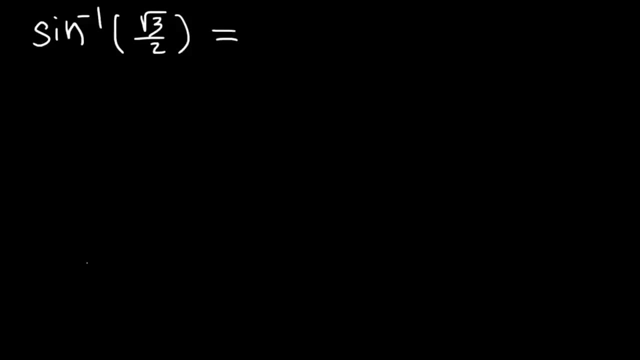 So go ahead and find the answer. Now we know that sine of- let's use degrees- Sine of 60 degrees- is equal to the square root of 3 over 2.. Also, sine of 300 is also root 3 over 2.. 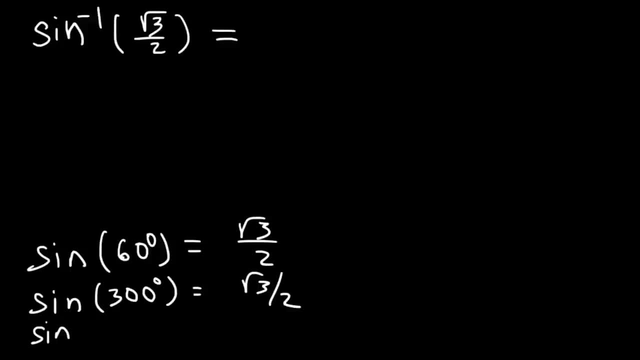 And at the same time I take that back. Sine of 300 is negative square root: 3 over 2.. Sine of 120 is positive root 3 over 2.. So we have two possible answers: 60 and 120.. 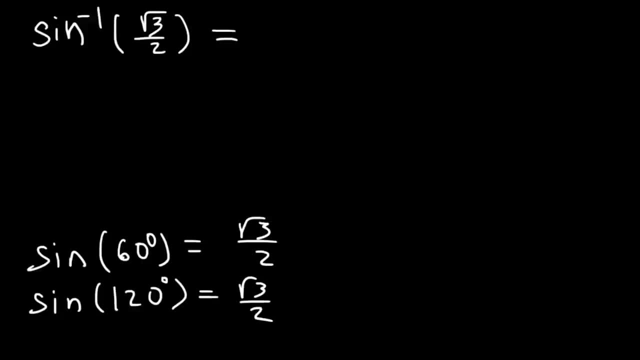 So which one should we use? Now? 60 is in quadrant 1,, which is okay. 120 is in quadrant 2.. And the arc sine function does not exist in quadrant 2.. So the answer is 60.. So the answer is 60.. 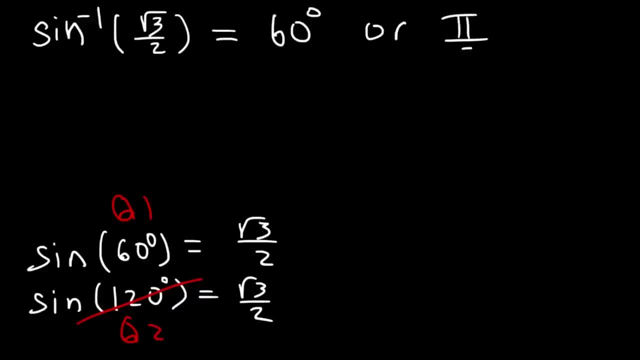 So the answer is 60 degrees, which we can write as pi over 3.. Keep in mind, pi is 180.. 180 divided by 3 is 60.. So that's the answer for this example. Arc sine of root, 3 over 2 is 60.. 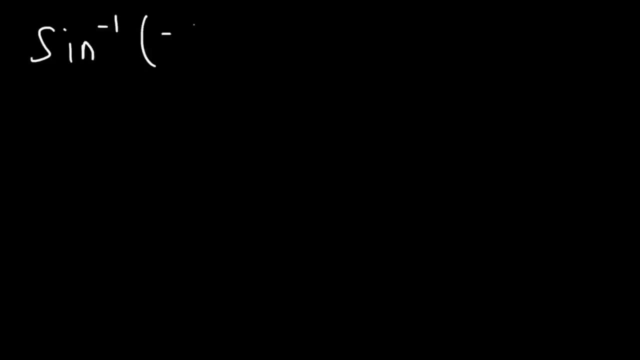 Now what about arc sine of negative 1 half? What's the answer for that? So sine of what angles is equal to negative 1 half? Let's make a list And then let's eliminate the wrongs. So we know: sine 30 is 1 half. 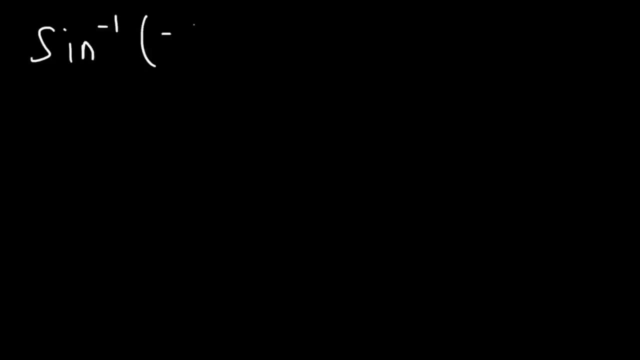 Now what about arc sine of negative 1 half? What's the answer for that? So sine of what angles is equal to negative 1 half? Let's make a list And then let's eliminate the wrongs. So we know: sine 30 is 1 half. 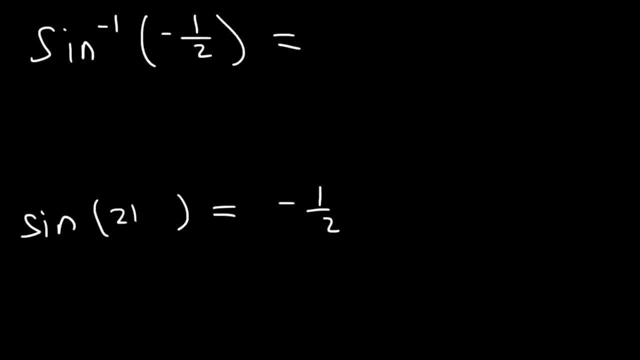 And sine 150 is 1 half. Sine 210 is negative 1 half. 210, 150, they all have a reference angle of 30. And 210 is in quadrant 3.. Sine of 330, which is in quadrant 4, that's also negative 1 half. 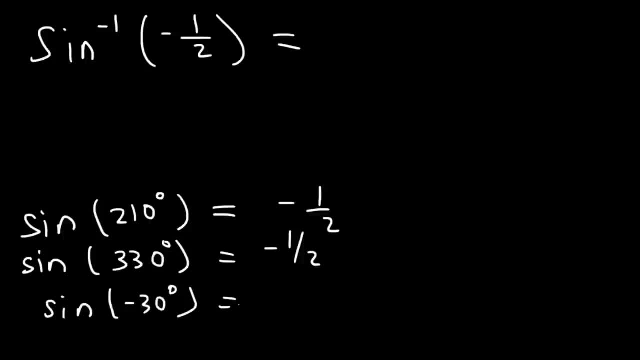 And also sine of negative 30,, that's in quadrant 4 as well. That's negative 1 half. So which one is the correct answer? So we know that the inverse sine function exists in quadrants 1 and 4. It does not exist in 2 and 3.. 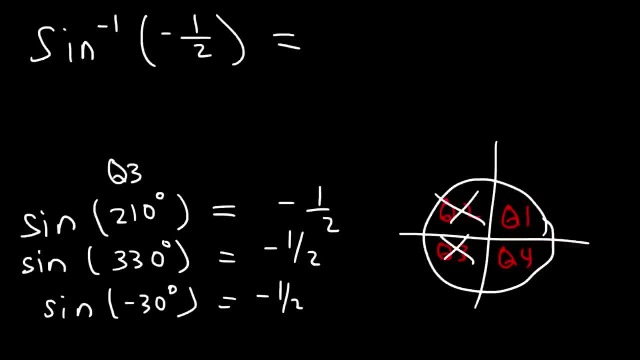 So 210 is in quadrant 3.. So that answer is eliminated. Now 330 is in quadrant 4. And negative 30 is also in quadrant 4.. So this is 330.. And this is negative 30. So which one is the answer? 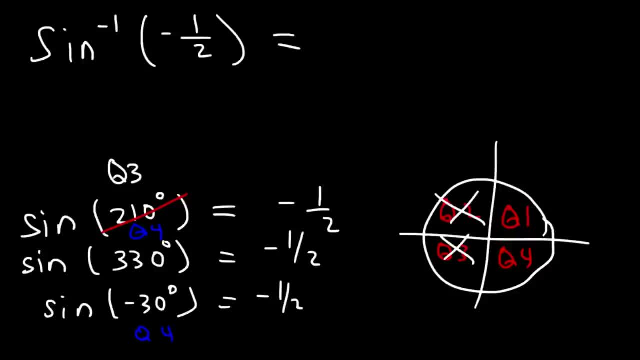 Because they both exist in the appropriate quadrant. Now don't forget about the range of the arc sine function. It's from negative pi over 2 to pi over 2.. Or negative 90 to positive 90.. 330 is not in that range. 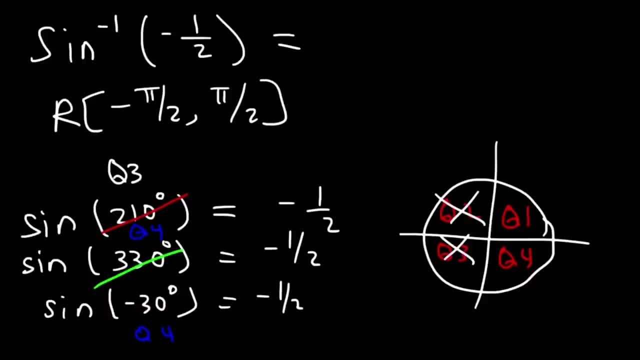 330 is the same as 11 pi over 6.. So your answer has to be between negative 90 degrees and 90 degrees. So this answer is within the appropriate range and it's in the right quadrant. So therefore, sine arc sine of negative 1, half is negative 30, or negative pi over 6.. 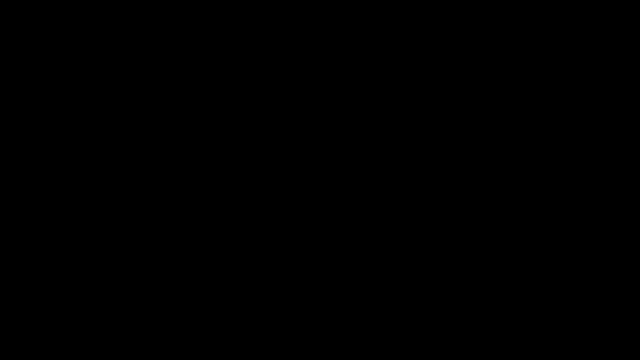 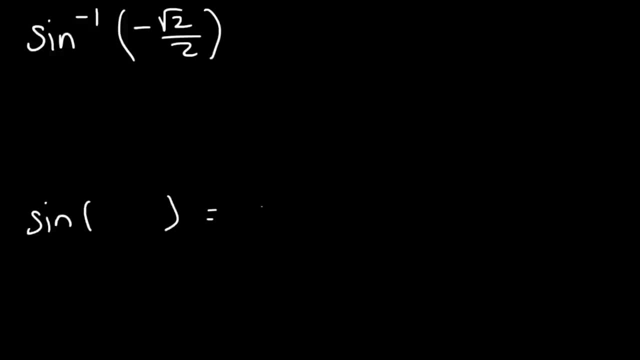 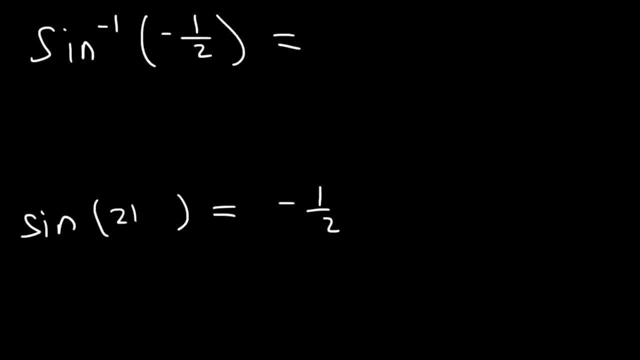 And sine 150 is 1 half. Sine 210 is negative 1 half. 210, 150, they all have a reference angle of 30. And 210 is in quadrant 3.. Sine of 330, which is in quadrant 4, that's also negative 1 half. 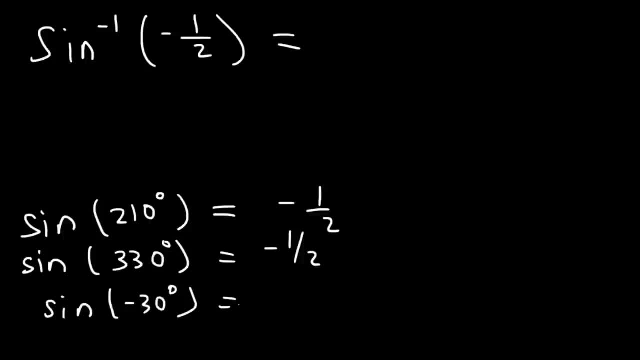 And also sine of negative 30,, that's in quadrant 4 as well. That's negative 1 half. So which one is the correct answer? So we know that the inverse sine function exists in quadrants 1 and 4. It does not exist in 2 and 3.. 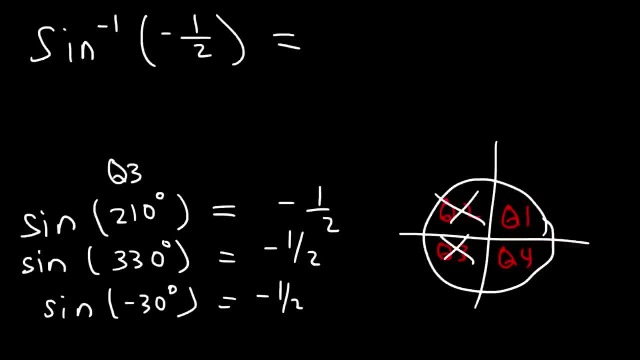 So 210 is in quadrant 3.. So that answer is eliminated. Now 330 is in quadrant 4. And negative 30 is also in quadrant 4.. So this is 330.. And this is negative 30. So which one is the answer? 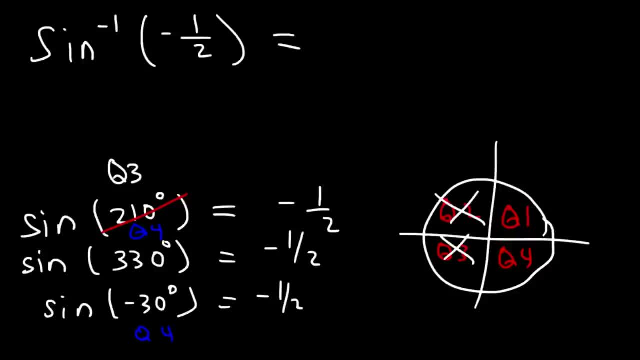 Because they both exist in the appropriate quadrant. Now don't forget about the range of the arc sine function. It's from negative pi over 2 to pi over 2.. Or negative 90 to positive 90.. 330 is not in that range. 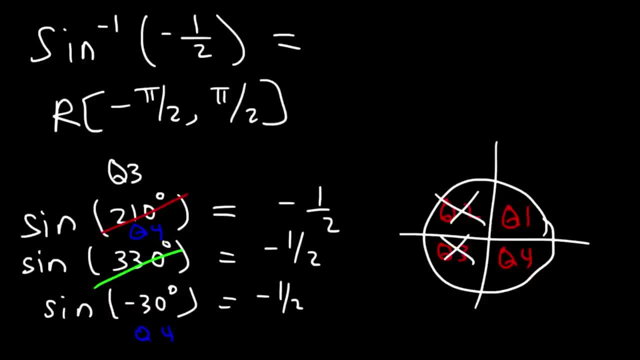 330 is the same as 11 pi over 6.. So your answer has to be between negative 90 degrees and 90 degrees. So this answer is within the appropriate range and it's in the right quadrant. So therefore, sine arc, sine, of negative 1, half is negative 30 or negative pi over 6.. 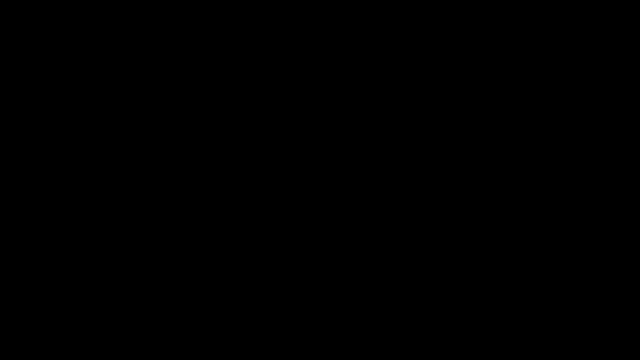 That's the answer that we want. Now let's work on another example. Go ahead and evaluate arc sine of negative square root, 2 over 2.. So sine of negative 1 half. So this is the answer. That's the answer that we want. 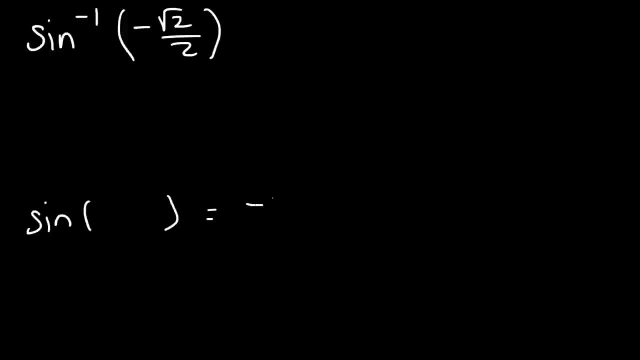 So sine of what angles is equal to negative root 2 over 2?? We know that sine 45 is equal to the square root of 2 over 2, but it's a positive answer, not a negative answer. Sine of 225 is equal to negative root 2 over 2, and sine of 315 is also equal to that. 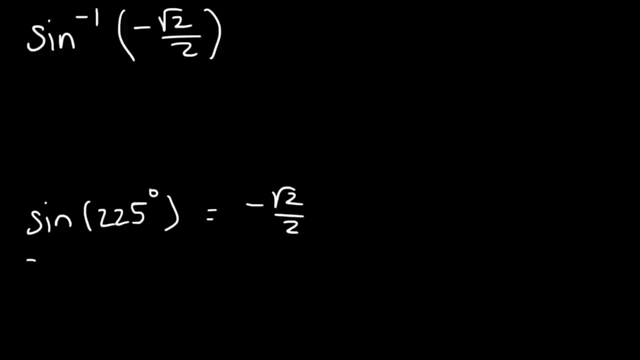 Sine of 225 is equal to negative root 2 over 2.. And sine of 315 is also equal to that. And the coterminal angle of 315, which is negative 45. Sine of negative 45 is equal to negative root 2 over 2.. 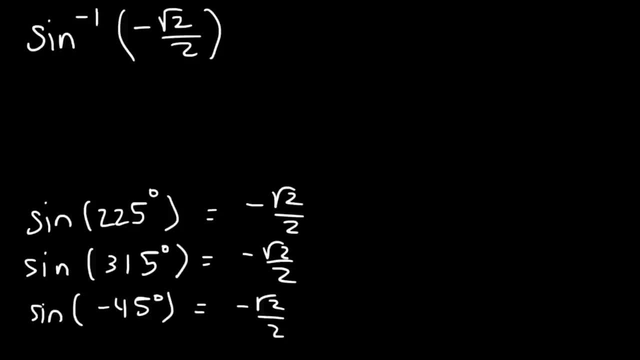 Now we're going to eliminate this answer because that's in quadrant 3. And the inverse sine function does not exist there. And we're going to eliminate this answer because it's not between negative 90 and 90. So this is the only answer that is within the range of negative 90 to 90 degrees and it's in quadrant 4.. 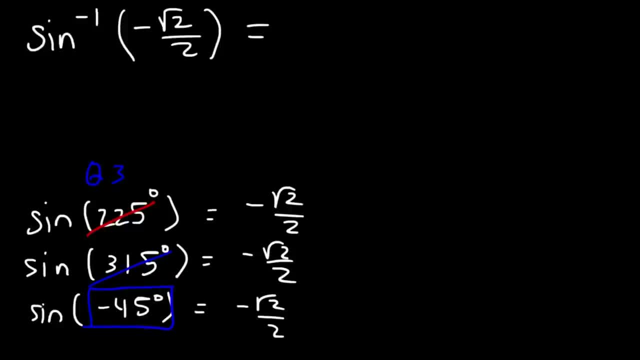 So arc sine of negative square root 2 over 2 is therefore equal to negative 45. Which is the same as negative pi over 4.. Now, what about these two? What is arc sine of 0,, arc sine of 1, and the inverse sine of negative 1?? 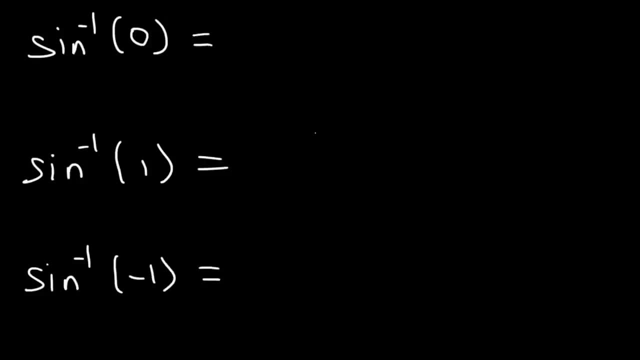 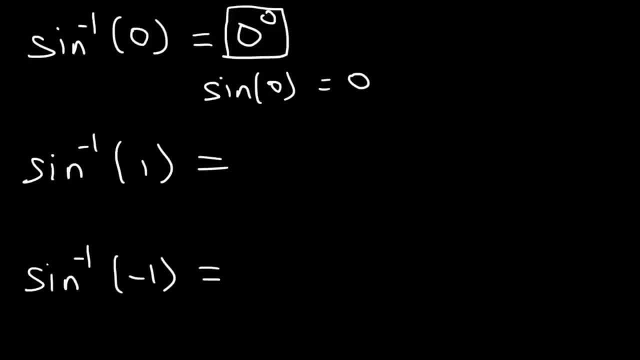 Then the range of negative pi over 2 to pi over 2.. Now arc sine of 1 is pi over 2.. So that's also in the range of the arc sine function. Arc sine of negative 1 is negative pi over 2.. 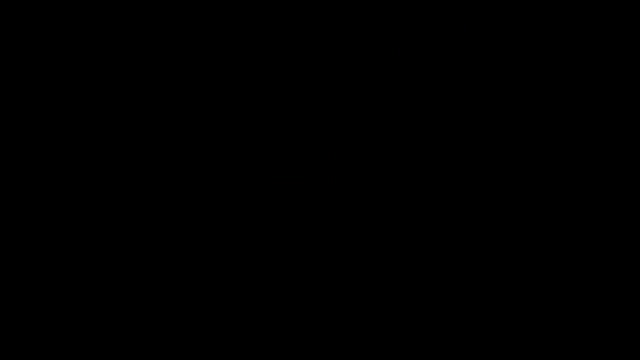 And so those are some other values that you want to be familiar with. Now let's move on to evaluating inverse cosine functions. So, let's evaluate inverse cosine functions. So what's the answer for this problem? Find the exact value of this function. 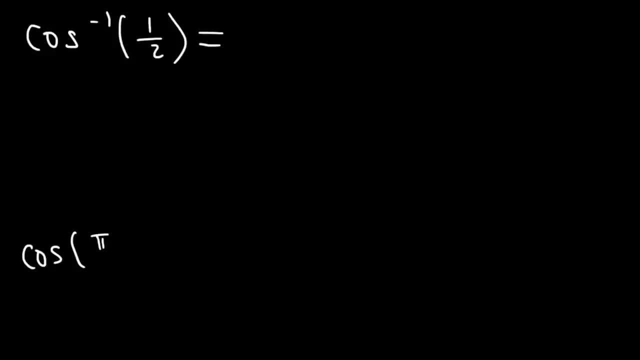 Well, we know that cosine of pi over 3,, that's cosine of 60 degrees, is equal to 1 half. Cosine of 5 pi over 3, which is in quadrant 4, is also equal to 1 half. 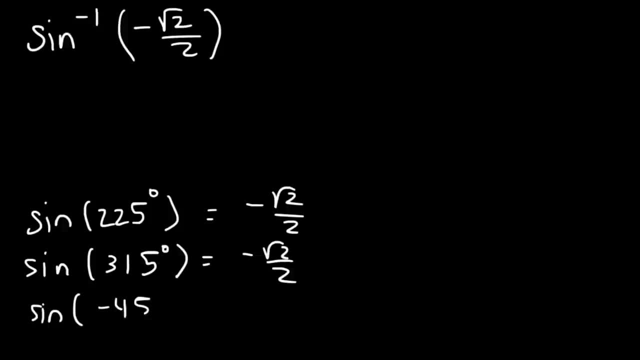 And the coterminal angle of 315, which is negative 45. Sine negative 45 is negative root 2 over 2.. Now we're going to eliminate this answer because that's in quadrant 3 and the inverse sine function does not exist there. 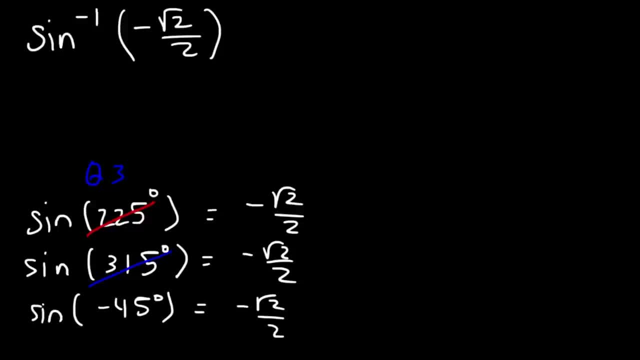 And we're going to eliminate this answer because it's not between negative 90 and 90.. So this is the only answer that is within the range of negative 90 to 90 degrees and it's in quadrant 4.. So arcsine of negative square root 2 over 2.. 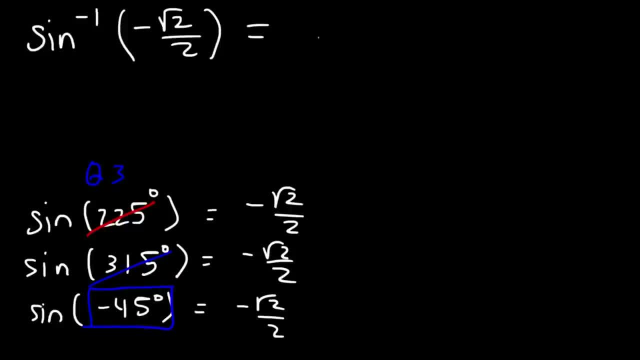 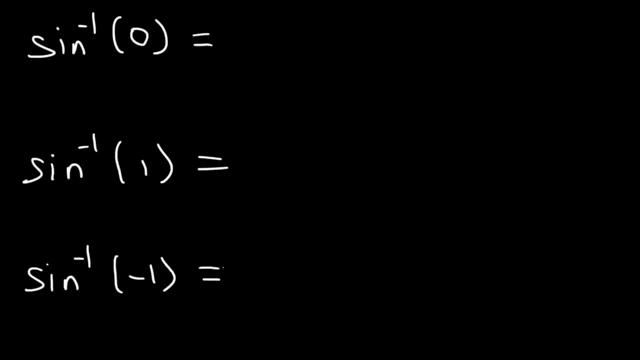 Is therefore equal to negative 45 degrees, which is the same as negative pi over 4.. Now, what about these two? What is arcsine of 0,, arcsine of 1, and the inverse sine of negative 1?? Find the values of these three things. 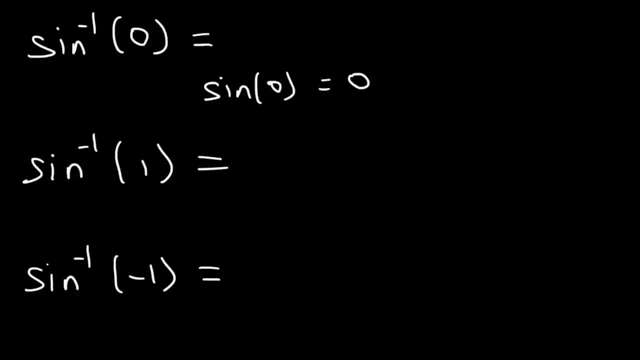 Now we know that sine of 0 is equal to 0. So this answer is 0 degrees, Zero degrees. it's within the range of negative pi over 2 to pi over 2.. Now arcsine of 1 is pi over 2.. 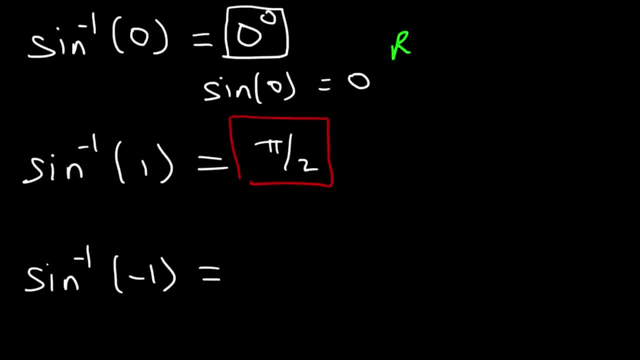 So that's also in the range of the arcsine function. Arcsine of negative 1 is negative pi over 2.. And so those are some other values that you want to be familiar with. Now let's move on to evaluating Inverse cosine functions. 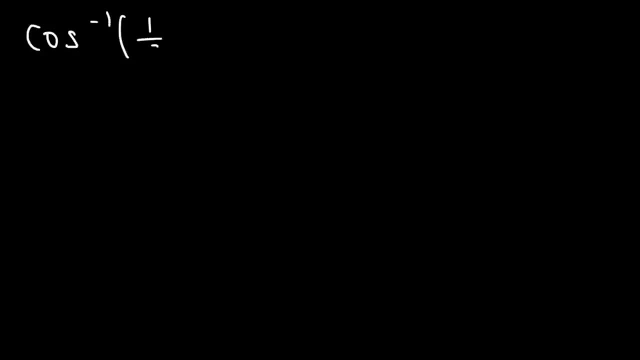 So let's evaluate inverse cosine 1 half. So what's the answer for this problem? Find the exact value of this function. Well, we know that cosine of pi over 3, that's cosine of 60 degrees, is equal to 1 half. 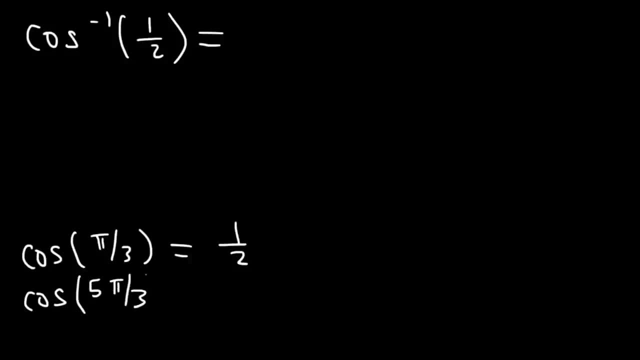 Cosine of 5 pi over 3, which is in quadrant 4, is also equal to 1 half Cosine is positive in quadrants 1 and 4, but negative in quadrants 2 and 3.. So which one is the answer? 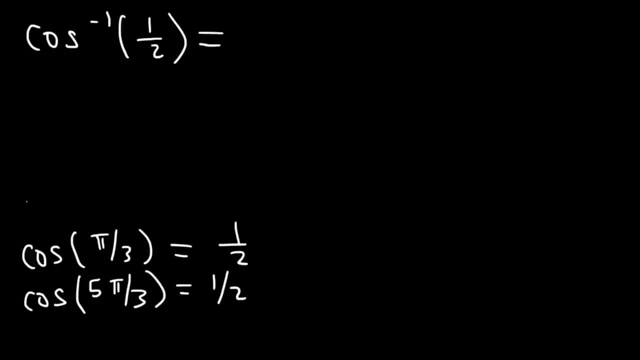 Is it pi over 3 or 5 pi over 3?? Now recall that the range of a cosine function, I mean of an arc cosine function, is from 0 to pi. So therefore arc cosine only exists in quadrants 1 and 2.. 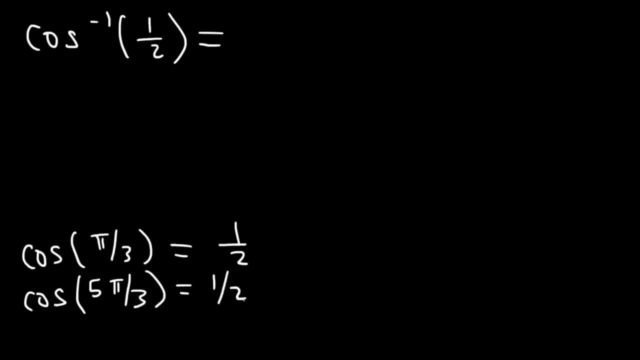 Cosine is positive in quadrants 1 and 4, but negative in quadrants 2 and 3.. So which one is the answer? Is it pi over 3 or 5 pi over 3?? Now recall that the range of a cosine function, I mean of an arc cosine function, is from 0 to pi. 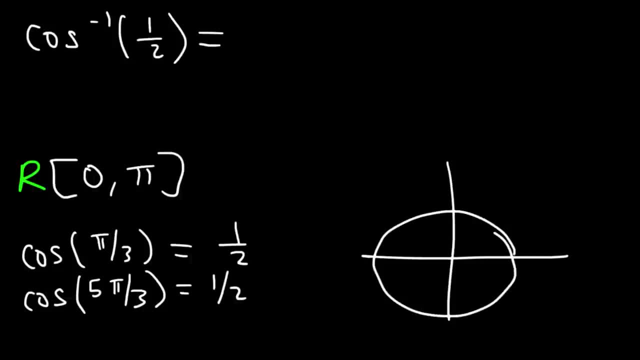 So, therefore, arc cosine only exists in quadrants 1 and 2.. So if you have a positive value, like what we do in this case, like what we have here, you want to make sure your angle is: if it's negative, it has to be between 90,, which is pi over 2, and 180,, which is pi. 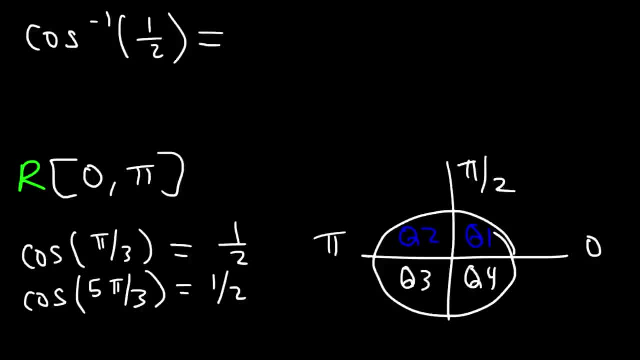 So cosine or arc cosine does not exist in quadrants 3 and 4.. So just keep that in mind. Therefore we can't use 5 pi over 3, that's in quadrant 4.. So arc cosine 1 half is equal to pi over 3, which is the same as 60 degrees. 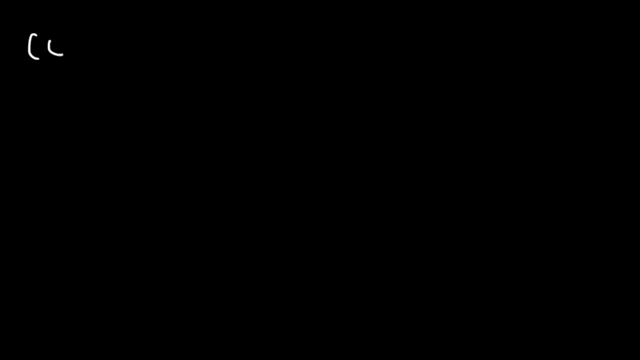 And so that's the answer. Now, what about this one? What is the inverse cosine of negative square root 3 divided by 2?? So take a minute and try that problem. Cosine of 30 degrees is positive square root 3 over 2, but we need a negative value. 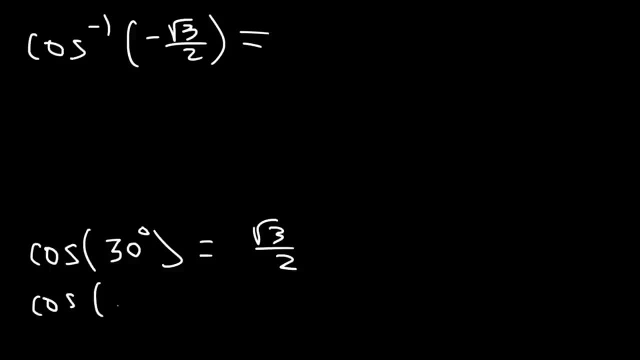 Cosine is negative in quadrants 2 and 3.. Cosine 150 is negative, root 3 over 2.. And cosine 210 is also negative, root 3 over 2.. We can eliminate 30 because it's not negative, it's positive. 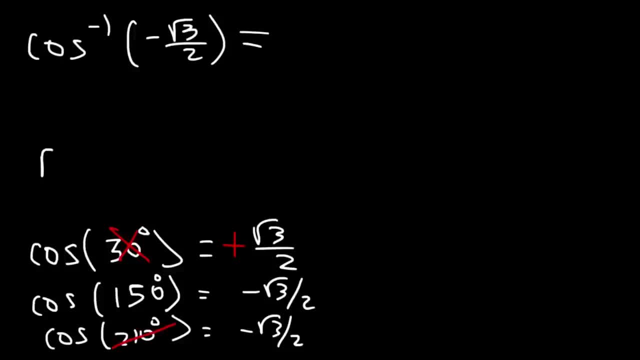 And we can eliminate 210 because it's not in the range of 0 to pi. 210 is in quadrant 3, and the arc cosine does not exist in quadrant 3.. 150,, on the other hand, is in quadrant 2.. 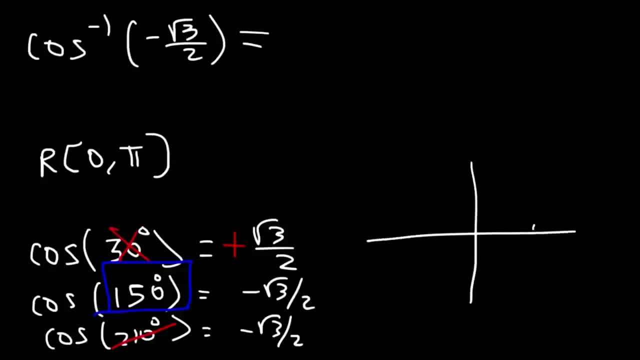 And the arc cosine function exists in quadrants 1 and 2, and also 150 is in the range it's between 0 and 180.. So 150 is the answer, which is the same as 5 pi over 6.. 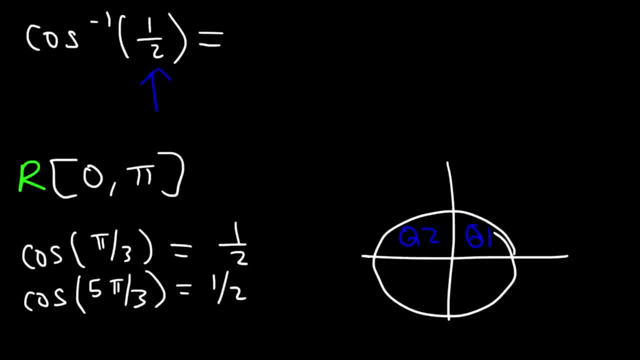 So if you have a positive value, Like what We do in this case, like what we have here, You want to make sure your angle is between 0 and 90.. If it's negative, it has to be between 90,, which is pi over 2, and 180,, which is pi. 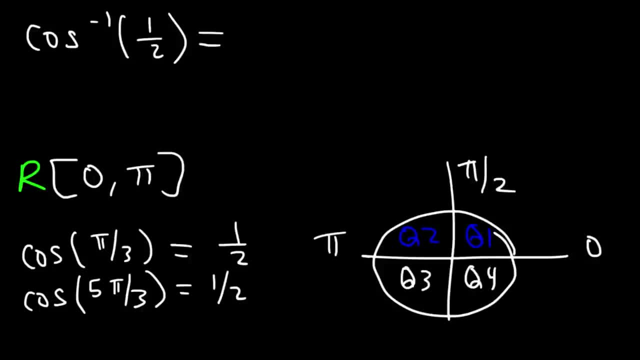 So cosine or arc cosine does not exist in quadrants 3 and 4.. So just keep that in mind. Therefore we can't use 5 pi over 3, that's in quadrant 4.. So arc cosine: 1 half. 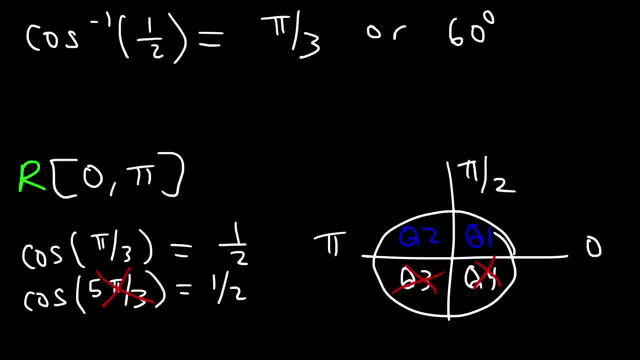 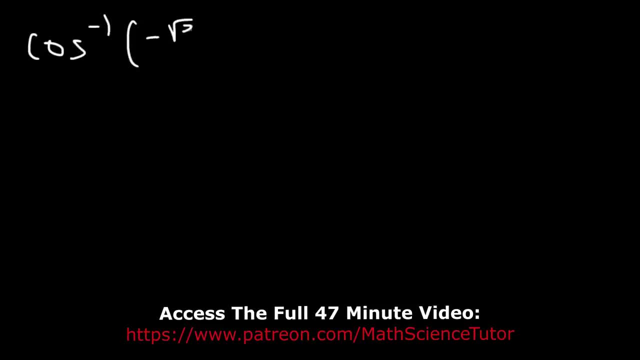 Is equal to pi over 3,, which is the same as 60 degrees, And so that's the answer. Now, what about this one? What is the inverse cosine of negative square root 3 divided by 2?? So take a minute and try that problem. 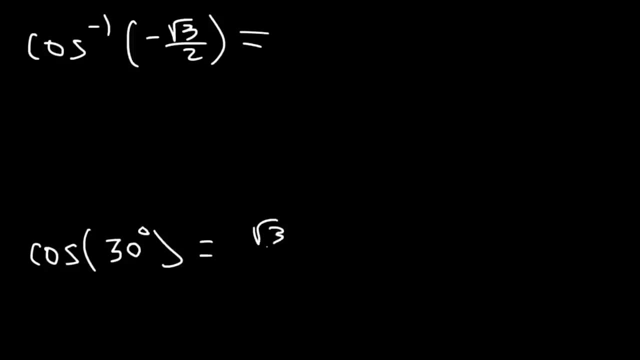 Cosine of 30 degrees is positive square root 3 over 2.. But we need a negative value. Cosine is negative in quadrants 2 and 3.. Cosine 150 is negative root 3 over 2.. And cosine 210 is also negative root 3 over 2.. 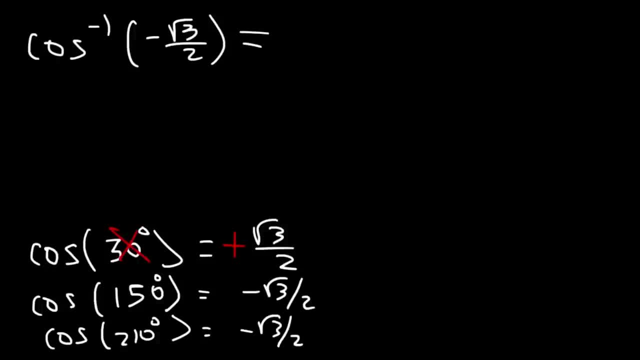 We can eliminate 30 because it's not negative, it's positive And we can eliminate 210 because it's not in the range of 0 to pi. 210 is in quadrant 3 and the arc cosine does not exist in quadrant 3.. 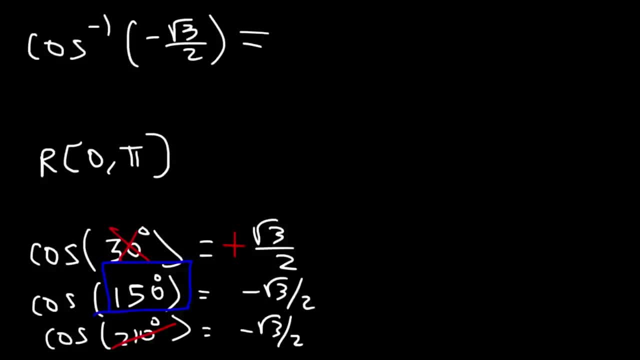 150, on the other hand, is in quadrant 2.. And the arc cosine function exists in quadrants 1 and 2.. And also 150 is in the range. It's between 0 and 180.. So 150 is the answer, which is the same as 5 pi over 6.. 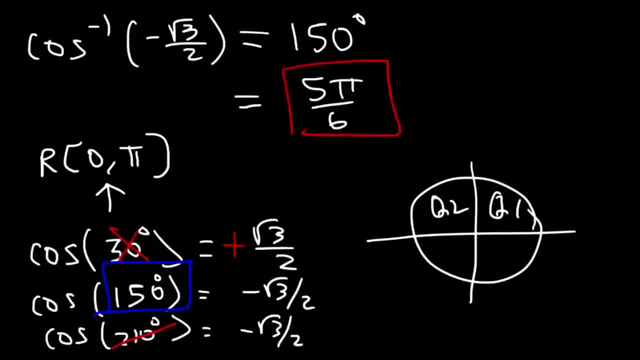 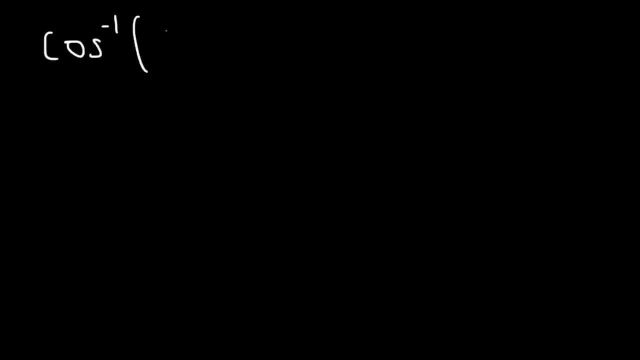 So arc cosine negative root 3 over 2 is equal to 5 pi over 6.. Go ahead and try this one: Arc cosine negative square root: 2 over 2.. So if you have a negative value, you need to choose the angle in quadrant 2.. 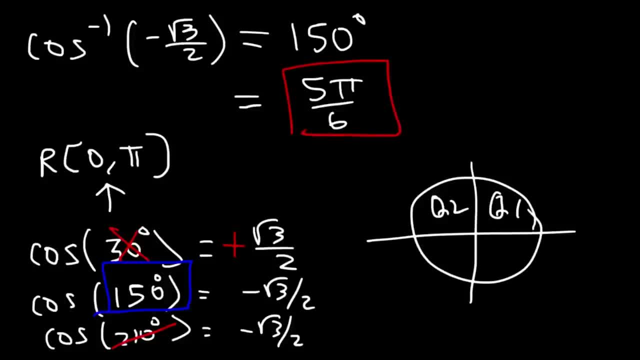 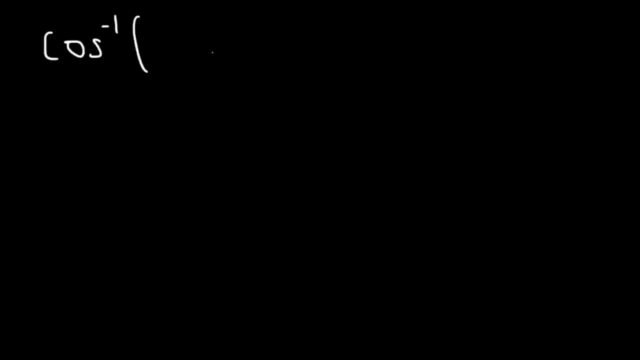 So arc cosine negative root 3 over 2 is equal to 5 pi over 6.. Go ahead and try this one: Arc cosine negative square root: 2 over 2.. So if you have a negative value, you need to choose the angle in quadrant 2.. 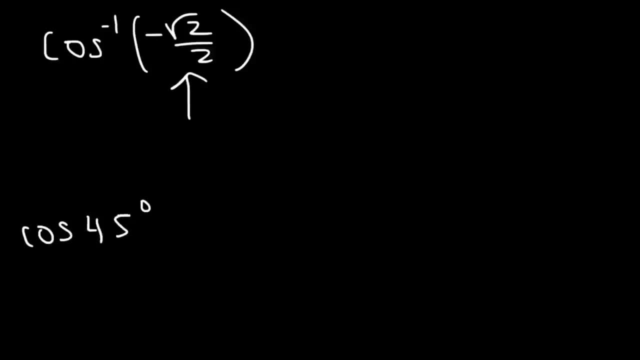 Now we know that cosine of 45 degrees is positive square root 2 over 2, but it's not negative. So, but this is the reference angle that we need In quadrant 2, the angle is 135, which has the same reference angle as 45.. 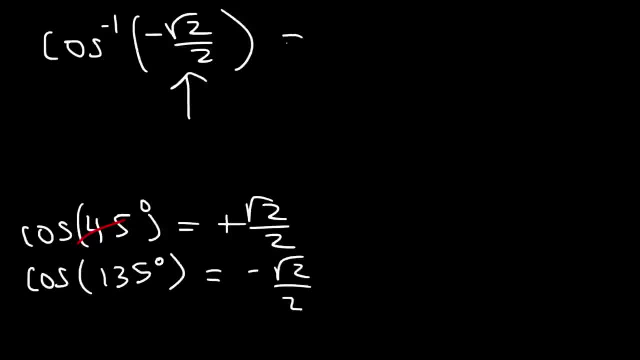 And this is negative square root 2 over 2.. So therefore, arc cosine negative root 2 over 2 is 135.. And this answer is In quadrant 2, it's between 0 and pi And this is the same as 3 pi over 4.. 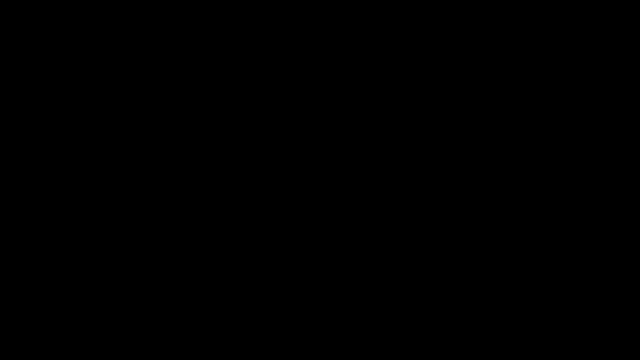 So that's the answer for this problem. Now go ahead and try these. This is arc cosine of 0,, arc cosine 1, and arc cosine negative 1.. And remember, the range is from 0 to pi. Now we know that cosine of pi. 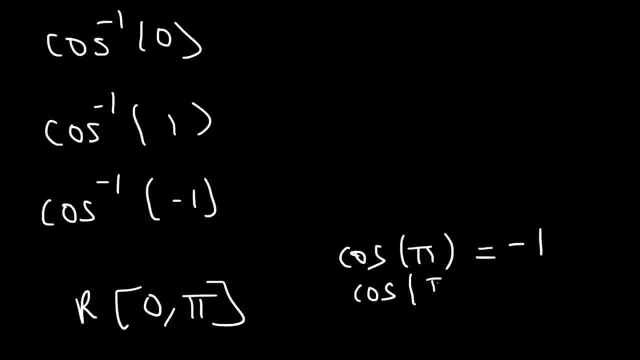 Is equal to negative. 1.. Cosine of pi over 2 is 0.. Cosine of 3 pi over 2 is 0. And cosine of 0 is 1.. So arc cosine of 0 must be pi over 2.. 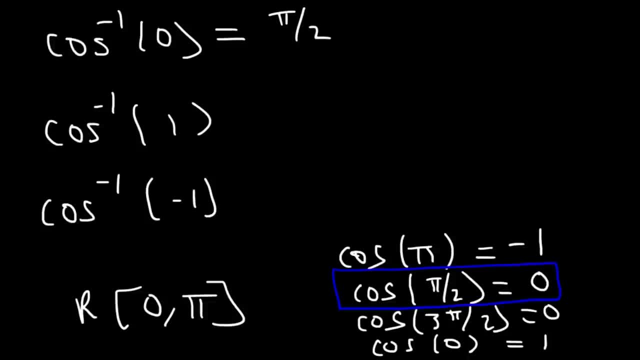 Based on this one here. If cosine pi over 2 is 0, arc cosine of 0 is pi over 2.. And pi over 2 is In the range. So that's the answer. Now, what about arc cosine of 1?? 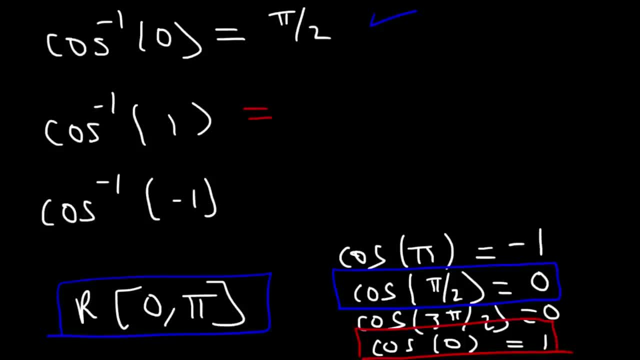 Well, cosine 0 is 1.. So therefore arc cosine 1 must be equal to 0. And 0 is included in the range, So that answer is acceptable. 3 pi over 2 is not between 0 and pi. 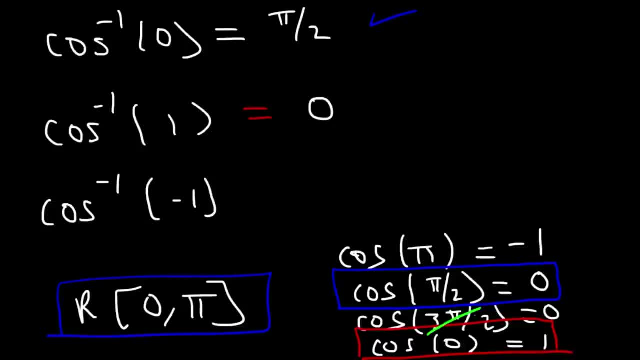 3. pi over 2 is 270 degrees. It's not between 0 and 180. So we can get rid of that one. Now pi is in the range If cosine pi Pi is equal to negative 1.. 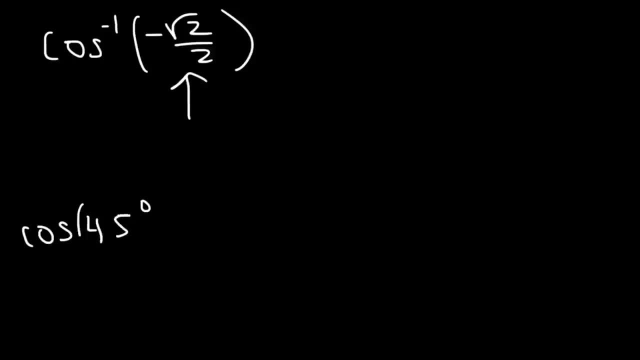 Now we know that cosine of 45 degrees is positive square root 2 over 2.. But it's not negative. But this is the reference angle that we need In quadrant 2, the angle is 135, which has the same reference angle as 45.. 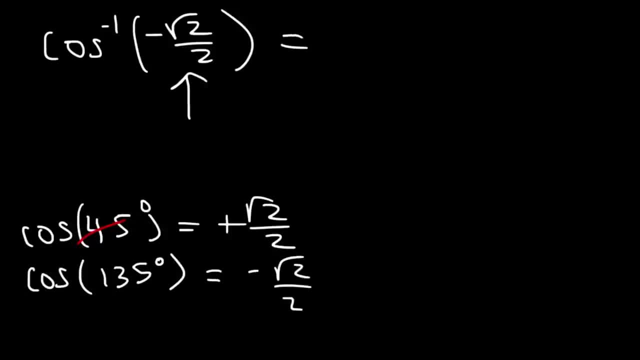 And this is negative square root 2 over 2.. So therefore, arc cosine negative root 2 over 2 is 135.. And this answer is in quadrant 2.. It's between 0 and pi And this is the same as 3 pi over 4.. 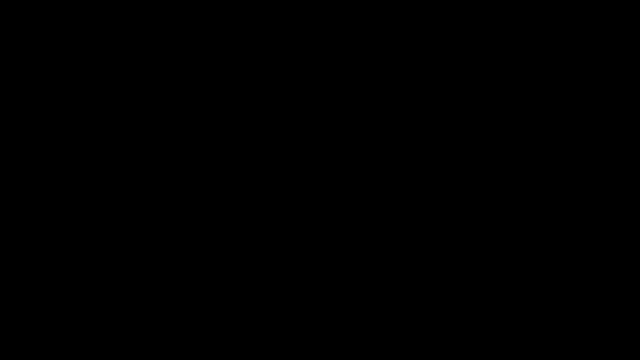 So that's the answer for this problem. Now go ahead and try these: Arc cosine of 0.. Arc cosine 1.. And arc cosine negative 1.. And remember the range is from 0 to pi. Now we know that cosine of pi is equal to negative 1.. 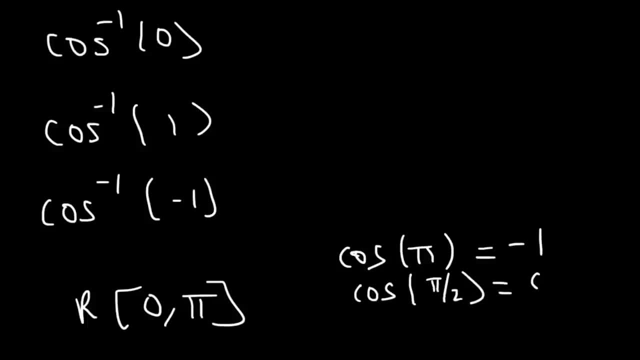 Cosine of pi over 2 is 0.. Cosine of 3, pi over 2 is 0.. And cosine of 0 is 1.. So arc cosine of 0 must be pi over 2.. Based on this one here. 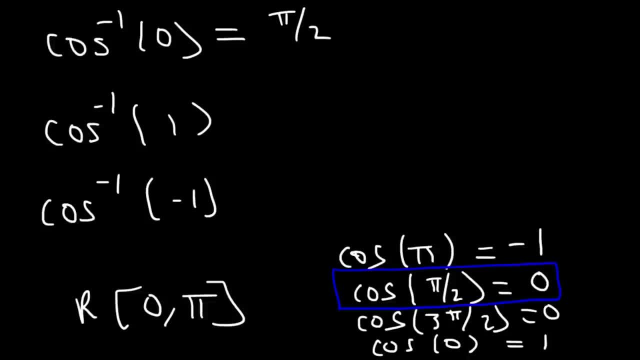 If cosine pi over 2 is 0, arc cosine of 0 is pi over 2.. And pi over 2 is within the range. So that's the answer. Now, what about arc cosine of 1?? Well, cosine 0 is 1.. 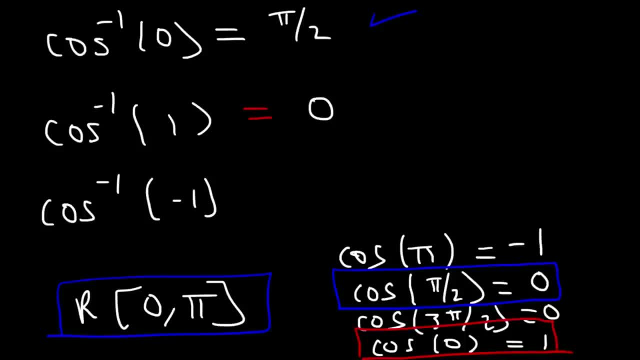 So therefore arc cosine 1 must be equal to 0. And 0 is included in the range, So that answer is acceptable. 3 pi over 2 is not between 0 and pi. 3 pi over 2 is 270 degrees. 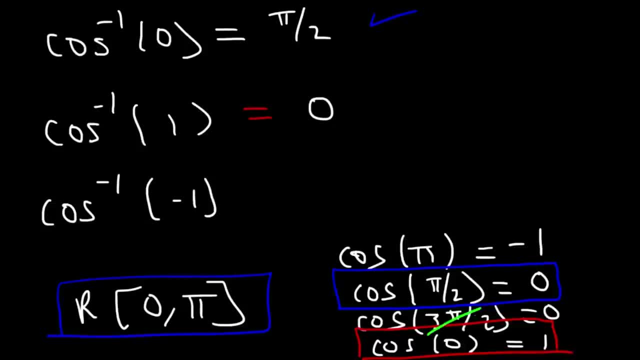 It's not between 0 and 180.. So we can get rid of that one. Now, pi is in the range. If cosine pi is equal to negative 1, arc cosine of negative 1 is pi. So these are the answers. 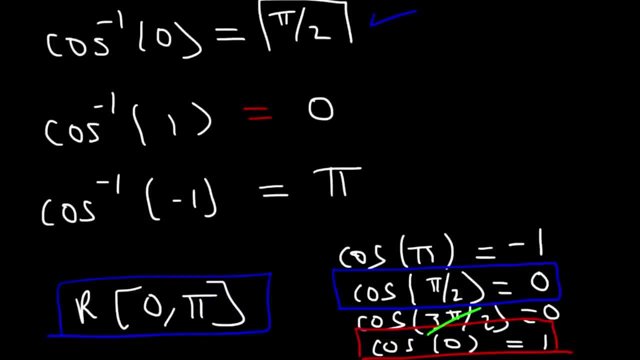 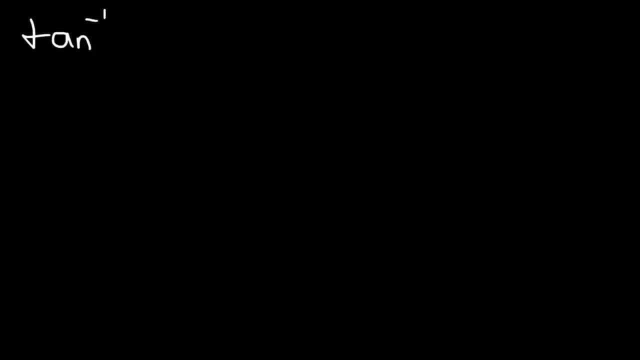 Arc cosine of negative 1 is pi. So these are the answers. Now let's talk about how to find the exact value of arc tangent functions. So let's start with the arc tangent of 0.. Tangent of what angle is equal to 0?? 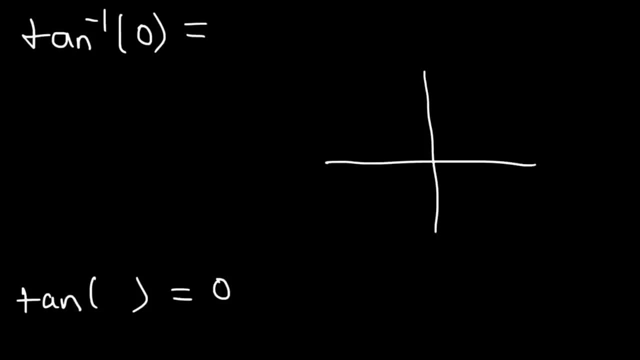 How can we figure this out? It turns out that tangent of 0 degrees is equal to 0. So here's how we know that. We know that tangent of an angle is equal to y over x, And at 0 degrees we have the point 1, 0. 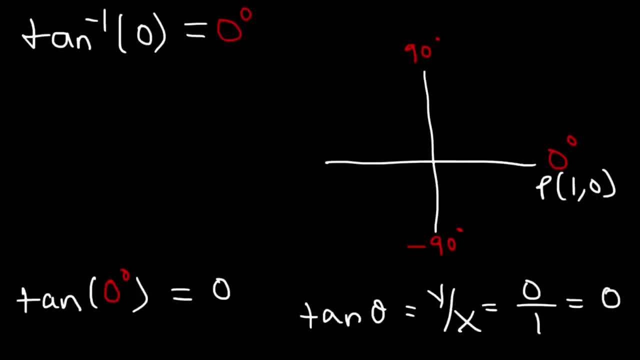 So y is 0, x is 1.. 0 divided by 1 is 0. So tangent of 0 degrees has a value of 0. So this is the angle And this is the value When dealing with inverse trig functions. 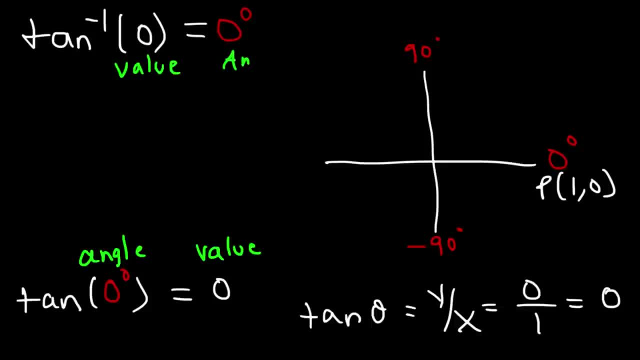 you have the value on the inside and you're looking for the angle. So the angle is 0 degrees. Now, what about this one? What is the inverse tangent of 1? What's the answer for that? So tangent of what angle is equal to 1?? 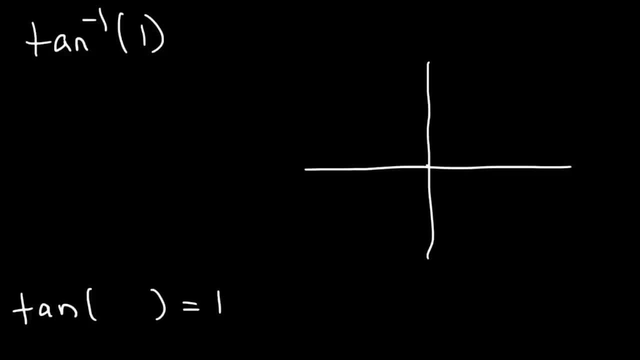 This occurs when y and x have the same value. At an angle of 45 degrees we have the point square root 2 over 2, comma square root 2 over 2.. So tangent of 45 is equal to y over x. 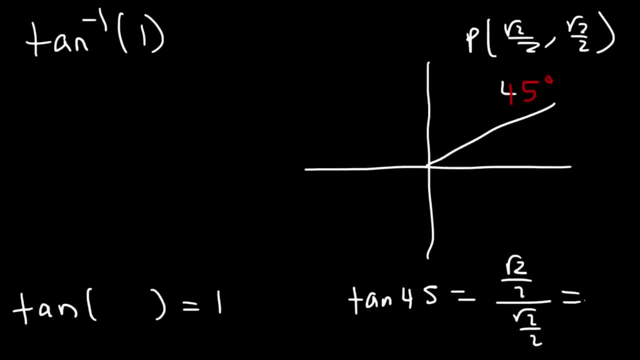 And whenever you divide two numbers that are the same, they will equal to 1.. So arc tangent of 1 is 45 degrees, which is the same. So that's the same as pi over 4.. That's the answer. 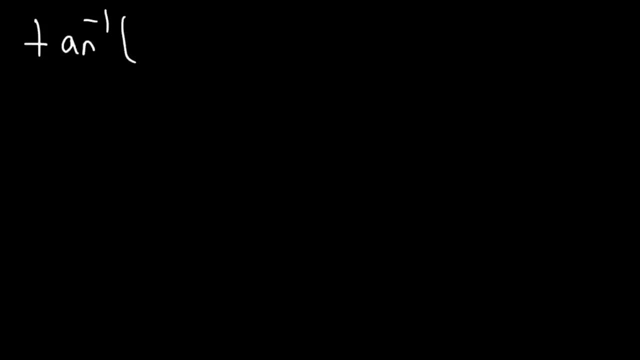 Now, if arc tangent of 1 is equal to pi over 4, what is the value of arc tangent of negative 1?? Now you need to know that the inverse tangent function has a range that's similar to the inverse sine function. 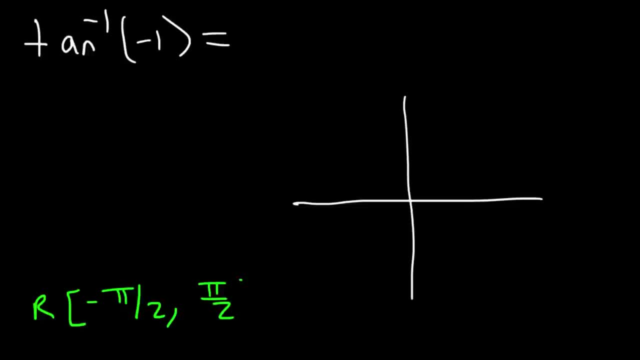 And that is from negative pi over 2 to pi over 2.. So if we were to draw the unit circle, the inverse tangent function, like the inverse sine function, exists only in quadrants 1 and 4. Between negative pi over 2 and pi over 2.. 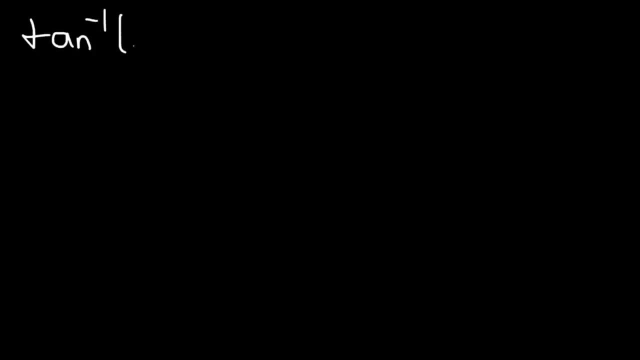 Now let's talk about how to find the exact value of arc tangent functions. So let's start with the arc tangent of 0.. Tangent of what angle is equal to 0? 0.. Let's figure this out. It turns out that tangent of 0 degrees is equal to 0.. 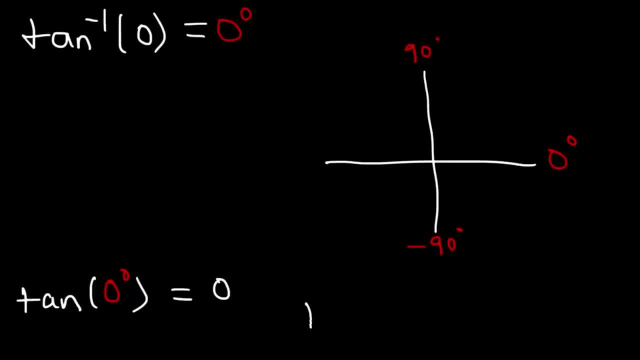 So here's how we know that. We know that tangent of an angle is equal to y over x, And at 0 degrees we have the point. So y is 0, x is 1, 0 divided by 1 is 0.. 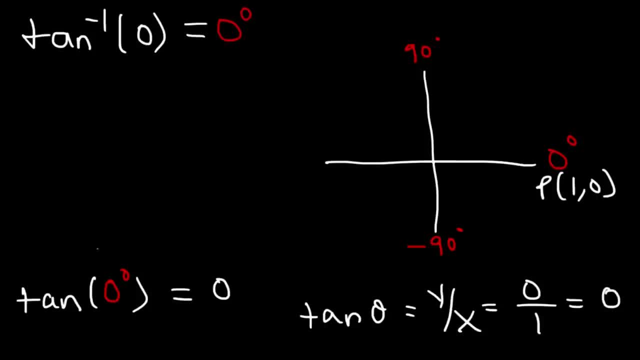 So tangent of 0 degrees has a value of 0.. 0. This is the angle and this is the value. When dealing with inverse trig functions, you have the value on the inside and you're looking for the angle. So the angle is 0 degrees. 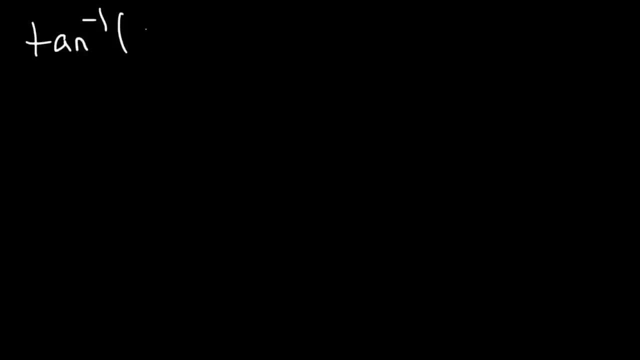 Now, what about this one? What is the inverse tangent of 1?? What's the answer for that? So tangent tangent of 0 degrees is 1.. Tangent of 1.. quindi, tangent of 0 degrees is 1.. So tangent of 0 is 1.. 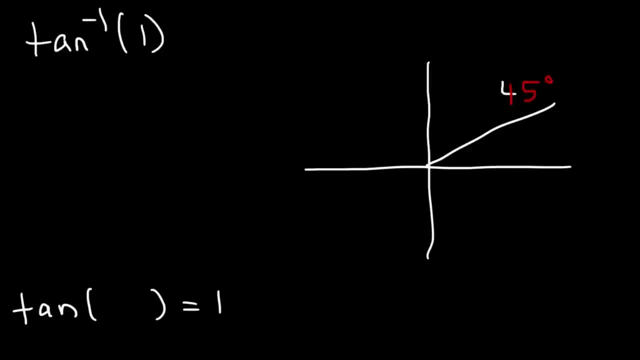 The answer is square root, 2 over 1.. So at this point you've learning the carbide equation. It's very simple. It's simple. The answer is tiver, and the solution is even Angle Angle of cube Y. 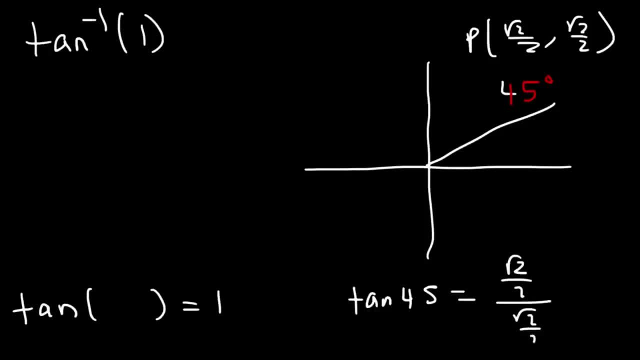 Angle of cube Y. Angle of cube Y. Angle of cube H. Angle of cube Z, they will equal to 1.. So arc tangent of 1 is 45 degrees, which is the same as pi over 4.. That's the answer. 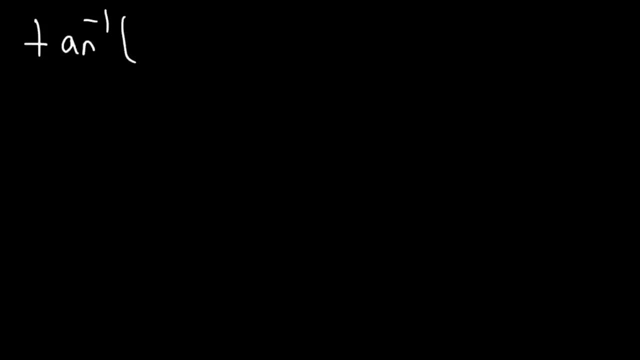 Now, if arc tangent of 1 is equal to pi over 4, what is the value of arc tangent of negative 1?? Now you need to know that the inverse tangent function has a range that's similar to the inverse sine function. 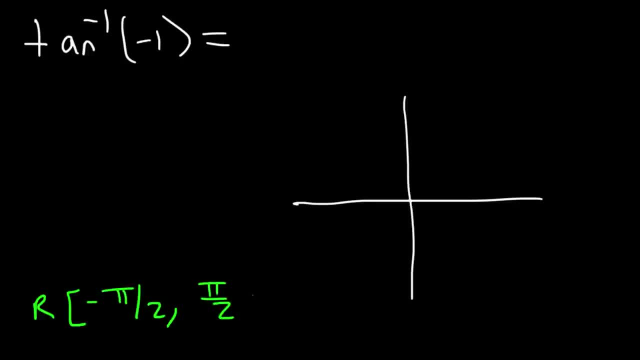 and that is from negative pi over 2 to pi over 2.. So if we were to draw the unit circle, the inverse tangent function, like the inverse sine function, exists only in quadrants 1 and 4, between negative pi over 2 and pi over 2.. 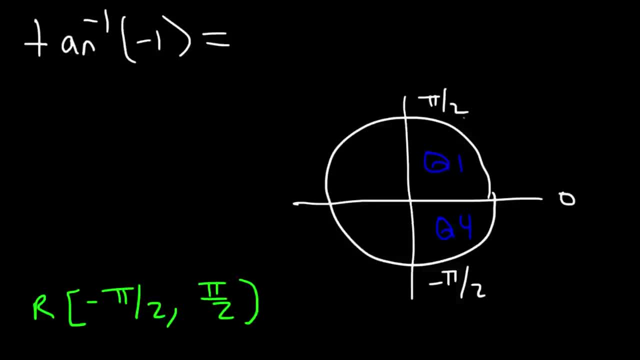 The inverse cosine function exists in quadrants 1 and 2, that is, between 0 and pi. So the only answer that's going to give us negative 1 is negative pi over 2.. The inverse sine function is at 45 degrees. 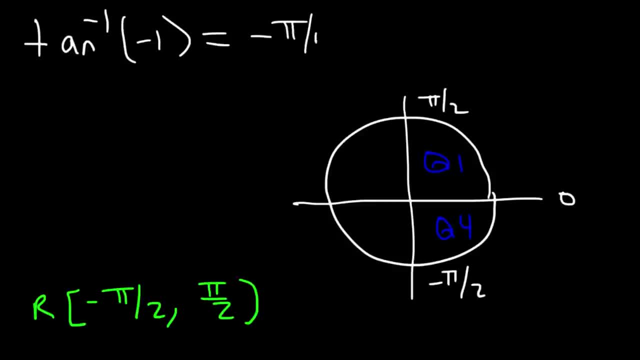 that is negative 45 in quadrant 4.. So this has to be negative pi over 4, which is in this region right here We can't use 7 pi over 4, because that's not in this range. So we have to use negative pi over 4.. 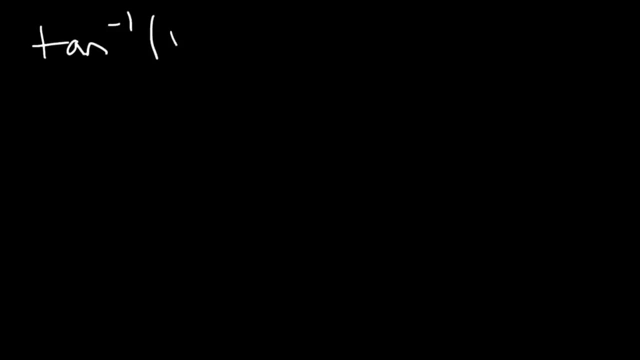 Now, what is the value of the inverse tangent of the square root of 3?? So, because we have a positive value, the answer has to be in quadrant 1.. So let's use the 30-60-90 reference triangle for this example. 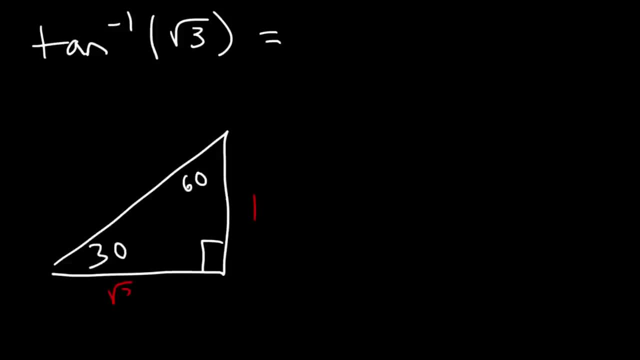 Across the 30 is 1, across the 60 is root 3, across the 90 is 2.. We know tangent is opposite over adjacent If we choose the 30 degree angle, opposite to it is 1,, adjacent to it is root 3.. 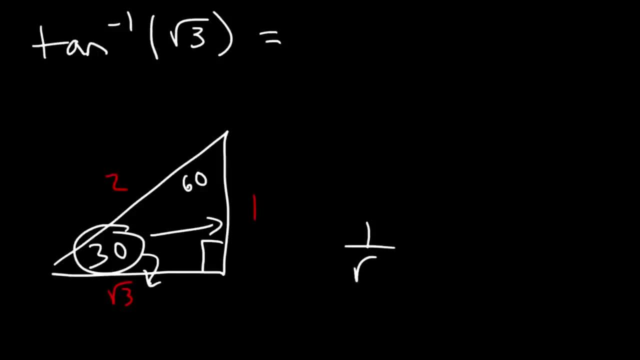 1 over root 3 is not the same as the square root of 3.. So, therefore, the angle that we have to use is 60.. Opposite to 60 is the square root of 3.. Adjacent to 60 is 1.. 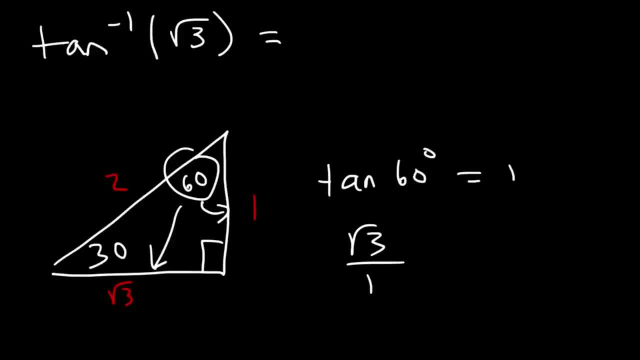 So tangent of 60 degrees is equal to the square root of 3.. So arctan of square root 3 is 60 degrees, or pi over 3, which is in quadrant 1.. If you get an answer in quadrant 1, it's okay. 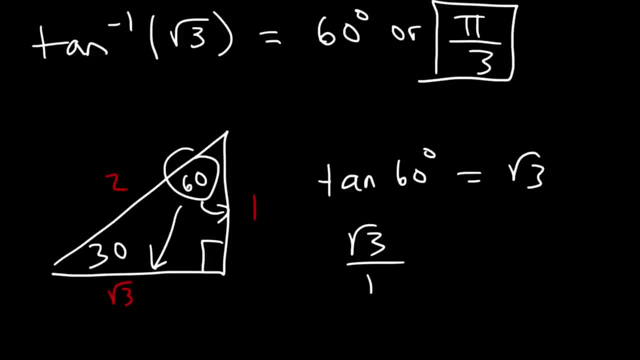 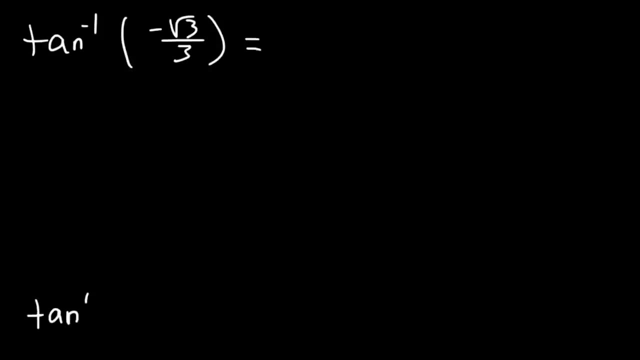 because arctan, arcsine, arccosine, they can all exist in quadrant 1.. Now what about the arctangent of negative square root 3 divided by 3?? What is that equal to? So tangent of what angle is equal to negative root 3 over 3?? 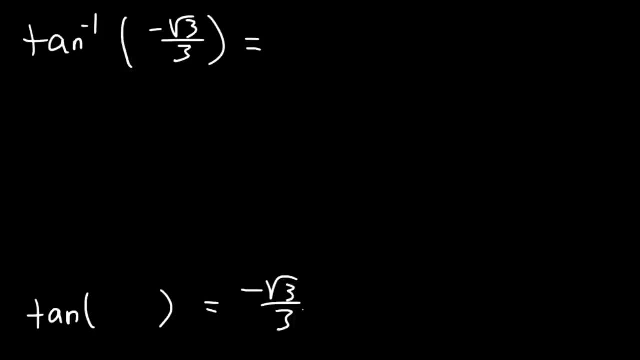 Now, if tangent 60 is the square root of 3, we know tangent 30 has to be root 3 over 3.. So 30 is the reference angle, but we need it to be in quadrant 4, so it's going to be negative 30.. 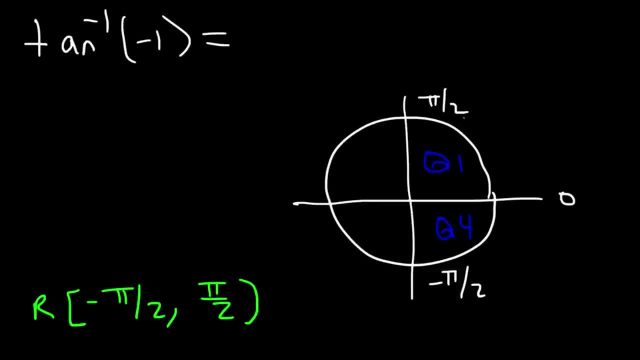 The inverse cosine function exists in quadrants 1 and 2. That is between 0 and pi. So the only answer that's going to give us negative 1 is at 45 degrees. That is, negative 45 in quadrant 4.. 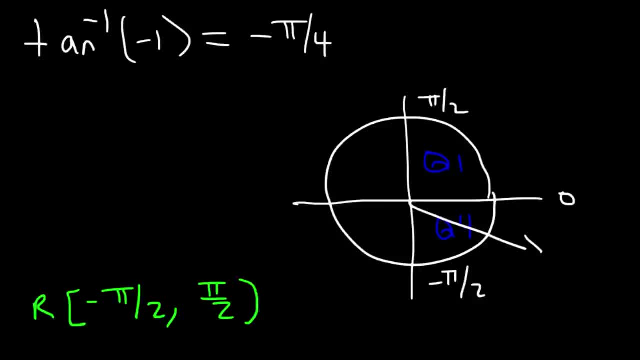 So this has to be negative pi over 4, which is in this region, right here We can't use 7 pi over 4 because that's not in this range, So we have to use negative pi over 4.. Now, what is the value of the inverse tangent? 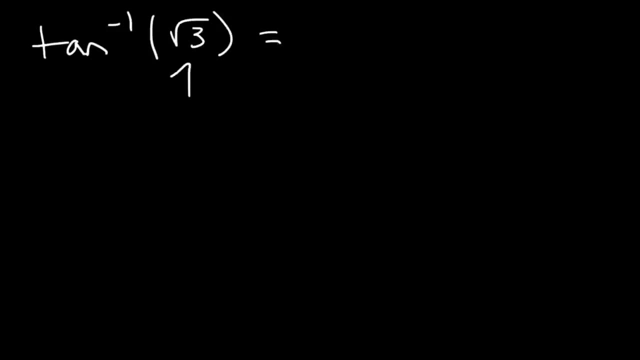 of the square root of 3?? So, because we have a positive value, the answer has to be in quadrant 1.. So let's use the 30-16-90 reference. Let's use the 30-16-90 reference triangle for this example. 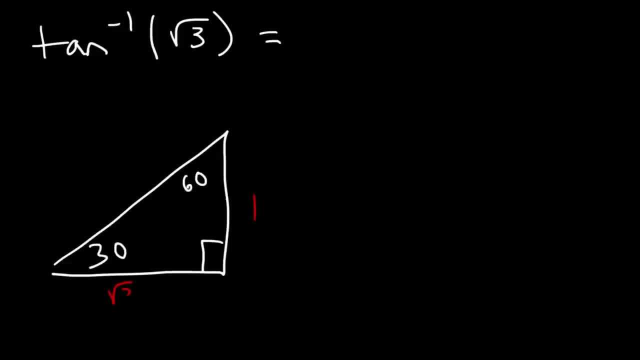 Across the 30 is 1.. Across the 60 is root 3. Across the 90 is 2.. We know tangent is opposite over adjacent. If we choose the 30-degree angle, opposite to it is 1., Adjacent to it is root 3.. 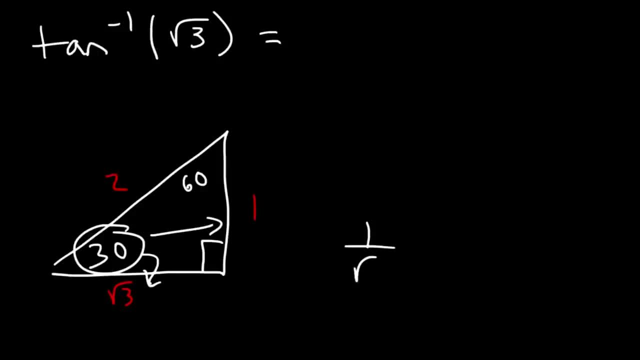 1 over root 3 is not the same as the square root of 3.. So, therefore, the angle that we have to use is 60.. Opposite to 60 is the square root of 3.. Opposite to 60 is the square root of 3.. 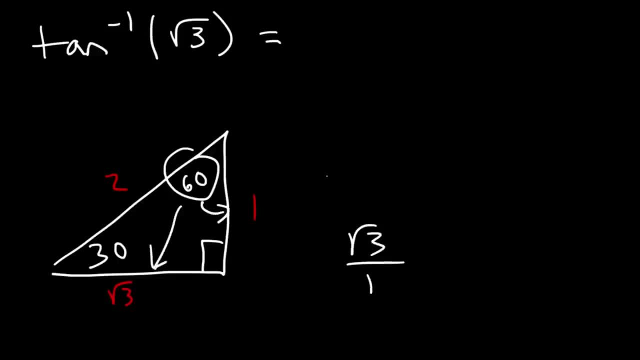 Opposite to 60 is the square root of 3.. Adjacent to 60 is 1.. So tangent of 60 degrees is equal to the square root of 3.. So arc tan of square root 3 is 60 degrees. 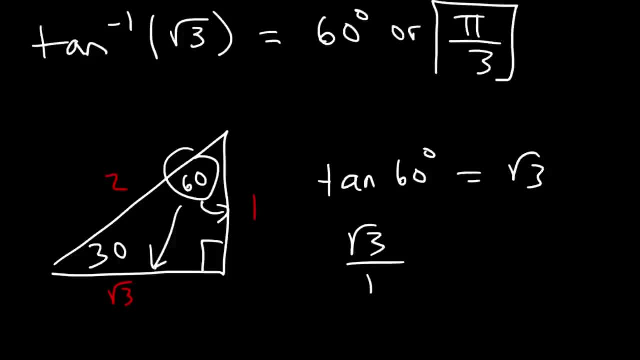 or pi over 3, which is in quadrant 1.. If you get an answer in quadrant 1, it's okay, Because arc tan, arc sine, arc cosine, they can all exist in quadrant 1.. Now, what about the arc tangent? 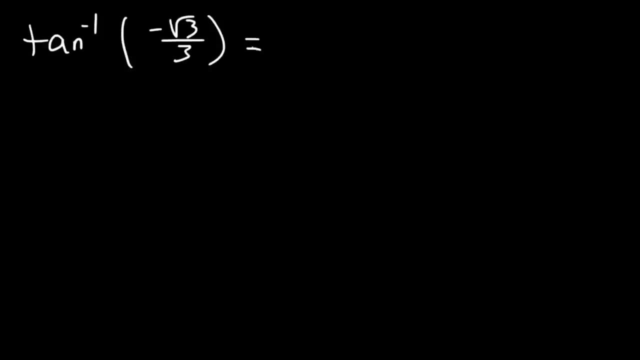 What about the arc tangent of negative square root 3 divided by 3?? What is that equal to? So tangent of what angle is equal to negative root 3 over 3?? Now, if tangent 60 is the square root of 3,? 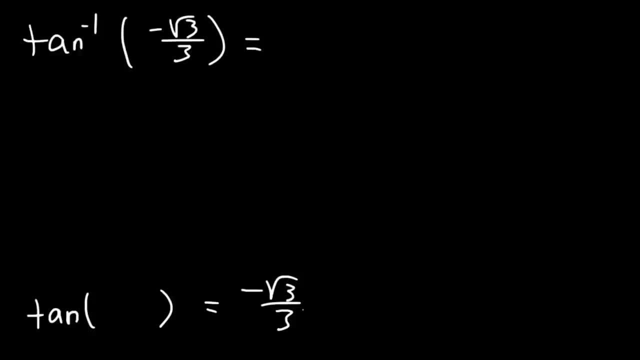 we know tangent 30 has to be root 3 over 3.. So 30 is the reference angle, but we need it to be in quadrant 4.. So it's going to be negative 30. We can confirm it. 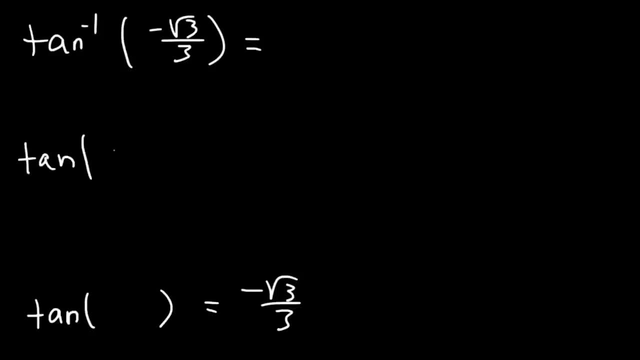 We can confirm it. So tangent of negative 30,, which is negative pi over 6, is equal to sine of negative pi over 6, or negative 30, divided by cosine of negative 30. Sine negative 30 is negative 1 half. 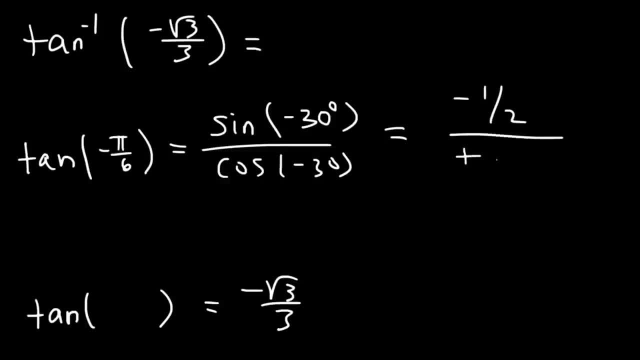 Sine is negative in quadrant 4, but cosine is positive, Cosine negative. 30 is root 3 over 2.. If we multiply the top and bottom by 2, we can get rid of these, And so we're left with negative 1 over the square root of 3.. 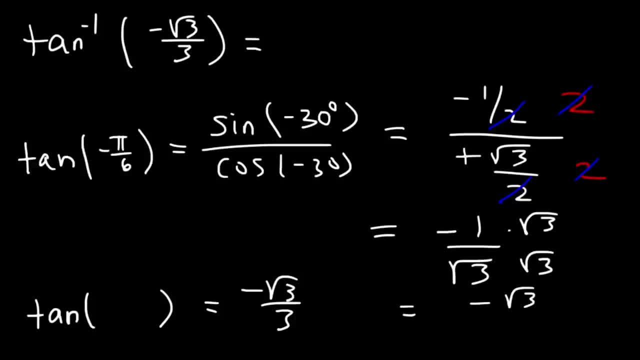 Now we have to rationalize it, So this becomes negative square root of 3 over 3.. Therefore, tangent of negative pi over 6 is equal to negative square root 3 over 3.. So the arctangent of negative root 3 over 3. 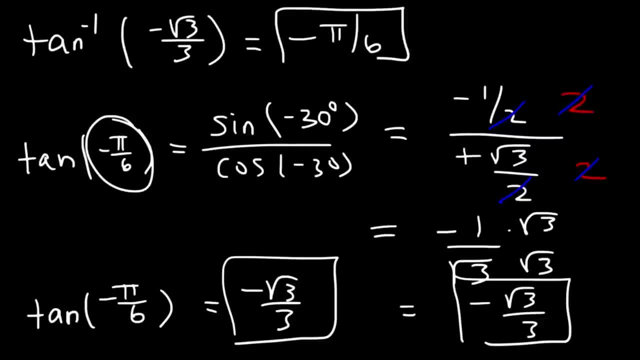 has to be negative pi over 6.. This exists in quadrant 4, and it's within the range of negative square root 3 over 3.. So this is negative pi over 2 to pi over 2.. So that's the answer. 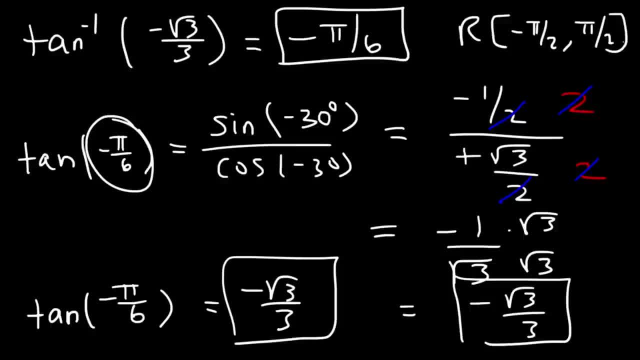 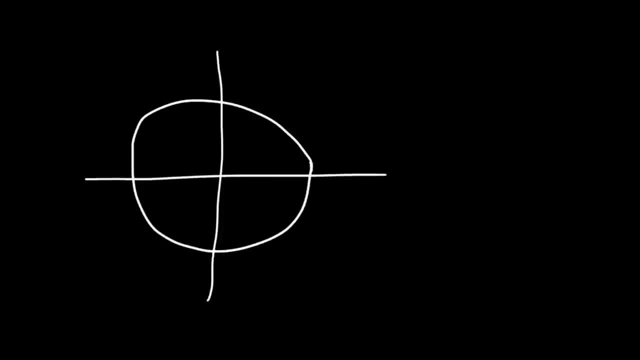 So now you know how to evaluate inverse trigonometric functions. So to review, remember this Arc cosine exists in quadrants 1 and 2. So that's with a range of 0 to pi. So as long as your answer is between 0 and pi, 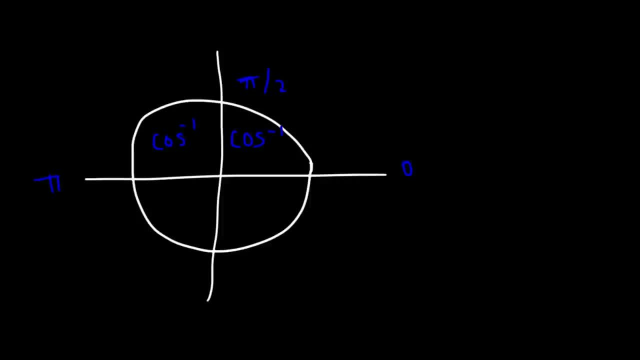 or within quadrant 1, you should be okay when evaluating arc cosine functions. The arc cosine function does not exist in quadrants 3 or 4.. So I'm just going to put an x in blue. Now for arc sine, which I'm going to use red. 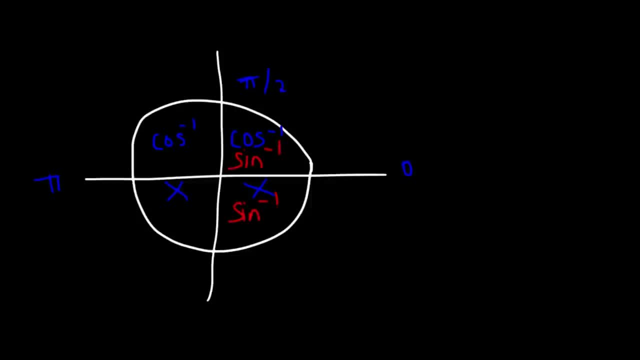 arc sine exists in quadrants 1 and quadrants 4. So that's within the range of negative pi over 2 to pi over 2. So arc sine does not exist in quadrants 2 and 3.. And then finally, 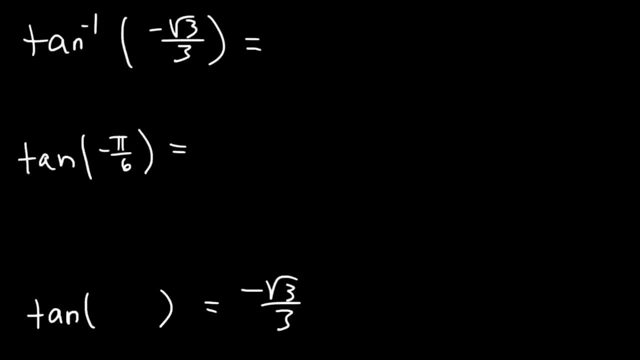 Tangent of negative 30, which is negative pi over 6, is equal to sine of negative pi over 6, or negative 30, divided by cosine of negative 30.. Sine negative 30 is negative 1 half Sine is negative in quadrant 4,. 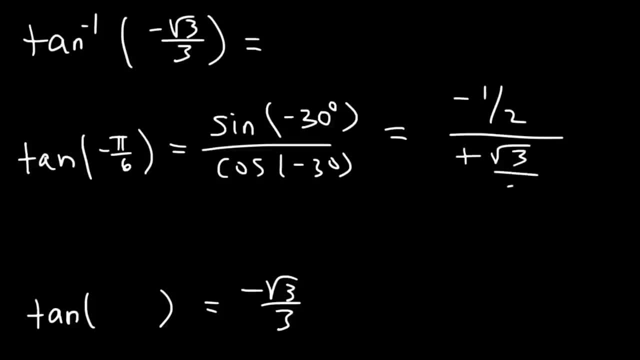 but cosine is positive, Cosine negative. 30 is root 3 over 2.. If we multiply the top and bottom by 2, we can get rid of these, And so we're left with negative 1 over the square root of 3.. 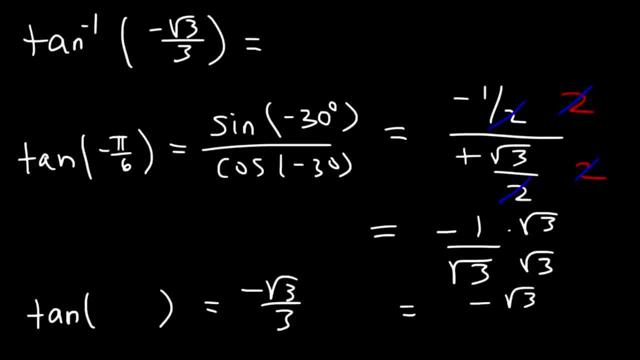 Now we have to rationalize it So this becomes negative square root of 3 over 3.. Therefore, tangent of negative pi over 6 is equal to negative square root 3 over 3.. So the arc tangent of negative root 3 over 3. 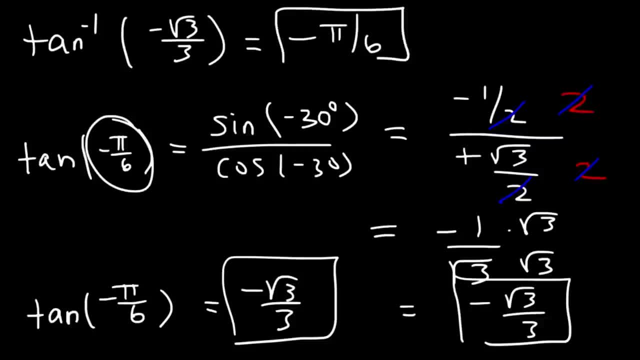 has to be negative pi over 6.. This exists in quadrant 4, and it's within the range of negative pi over 2 to pi over 2.. So that's the answer. So now you know. Now you know how to evaluate inverse trigonometric functions. 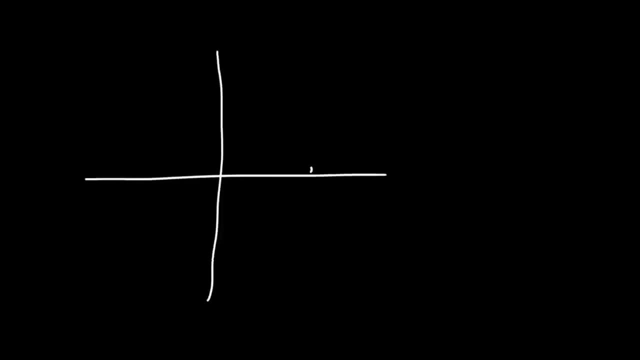 So to review, remember this Arc cosine exists in quadrants 1 and 2. So that's with a range of 0 to pi. So as long as your answer is between 0 and pi or within quadrant 1 and 2,. 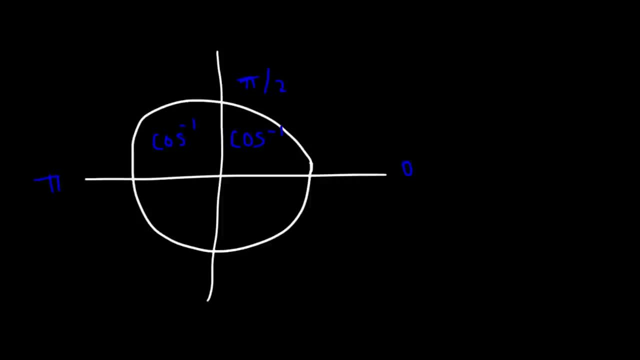 you should be okay when evaluating arc cosine functions. The arc cosine, the arc sine function does not exist in quadrants 3 or 4.. So I'm just going to put an x in blue Now for arc sine, which I'm going to use red. 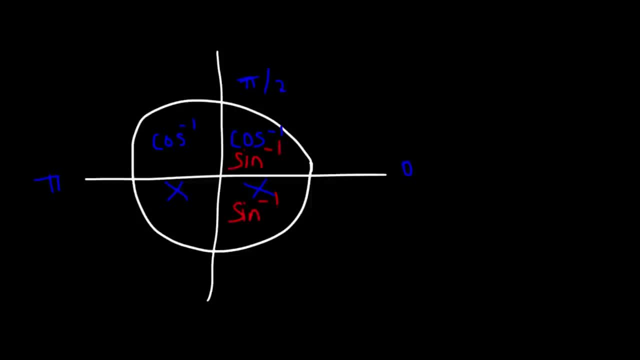 arc sine exists in quadrants 1 and quadrants 4.. So that's within the range of negative pi over 2 to pi over 2.. So arc sine does not exist in quadrants 1 and quadrants 2.. 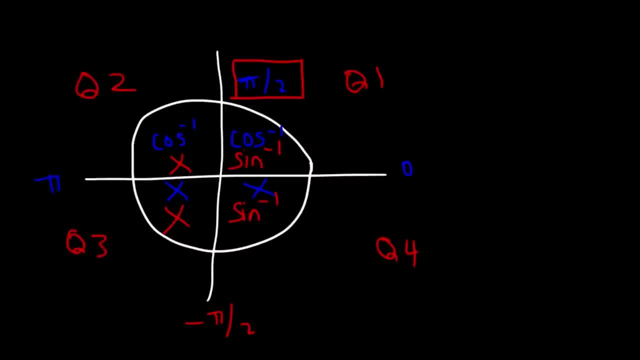 So arc sine does not exist in quadrants 2 and 3.. And then, finally, arc tangent is the same for arc sine, So arc tan exists in quadrants 4 and 1.. And that is between negative pi over 2 and pi over 2.. 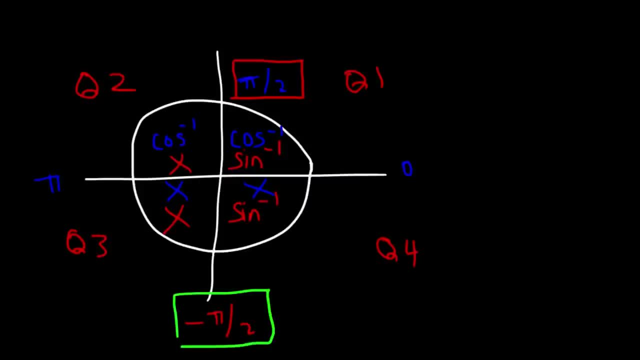 arc tangent is the same for arc sine. So arc tan exists in quadrants 4 and 1. And that is between negative pi over 2 and pi over 2.. It does not exist in 2 and 3.. None of them exist in quadrant 3,. 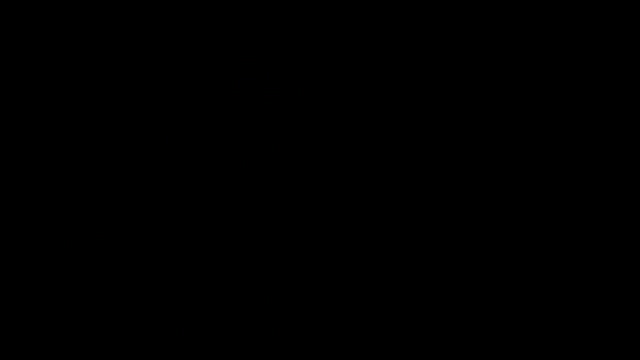 so you should never use an angle there. So remember arc cosine has a range of 0 to pi, So your answer has to be in that range. For arc sine and arc tangent, when getting an answer it has to be between negative pi over 2. 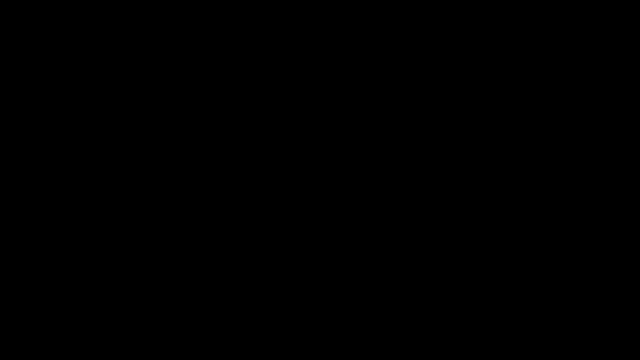 and pi over 2.. Now let's say if we have a composition of an inverse trait function, What should we do? So, for example, let's say, if we want to evaluate arc sine of sine, pi over 3.. What's the answer? 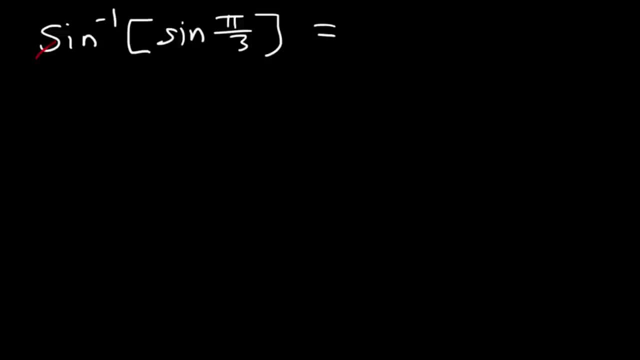 For this particular example, it turns out that arc sine and sine will cancel giving us an answer of pi over 3.. And we can do that because pi over 3 is in quadrant 1.. And arc sine exists in quadrant 1.. 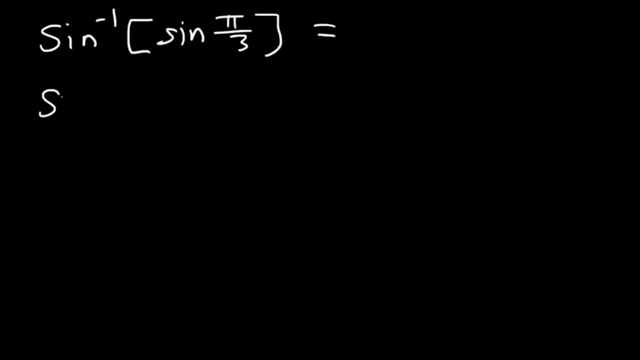 But let's take it one step at a time. So first let's evaluate sine pi over 3. Or sine 60 degrees. So using the unit circle or using the 30-60-90 reference triangle, you know that sine of 60. 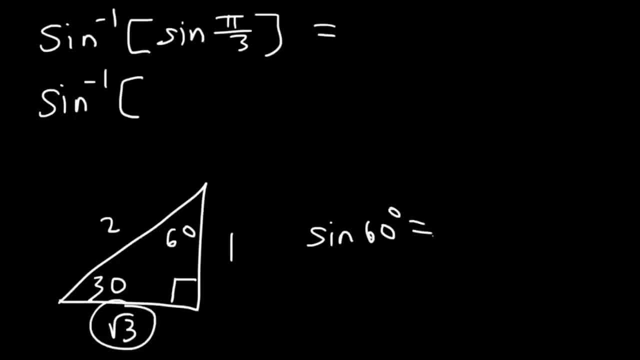 is equal to the opposite side, which is square root 3, divided by the hypotenuse 2.. So sine 60, or sine pi over 3, is the square root of 3 over 2.. Now we need to evaluate arc sine. 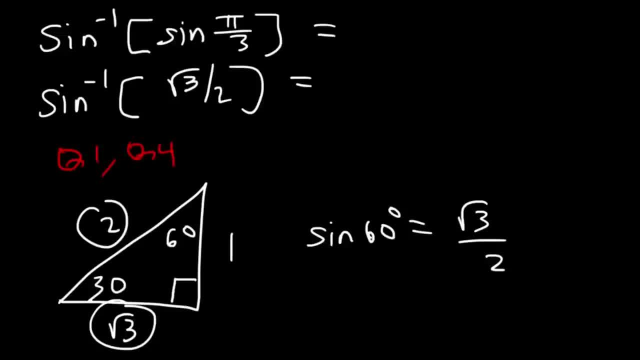 Arc sine exists in quadrants 1 and 4.. Now, because this is positive, we don't want the answer in quadrant 4, because arc sine is negative in quadrant 4.. So, therefore, the angle has to be 60.. It's going to be pi over 3. 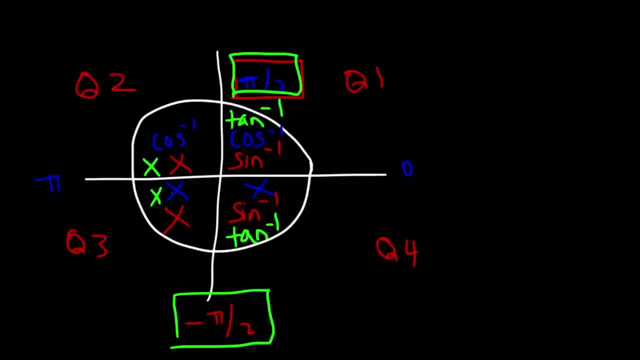 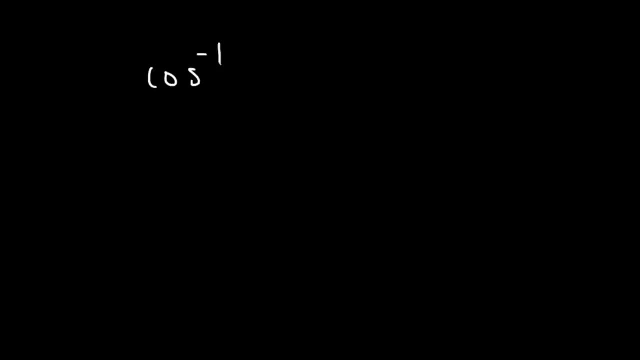 It does not exist in 2 and 3. None of them exist in quadrant 3. So you should never use an angle there. So remember, arc cosine has a range of 0 to pi, So your answer has to be in that range. 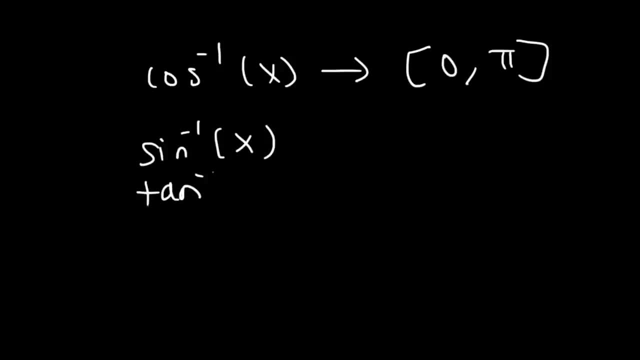 For arc sine and arc tangent. when getting an answer, it has to be between negative pi over 2 and pi over 2.. Now let's say if we have a composition of an inverse trait function, What should we do So? for example, 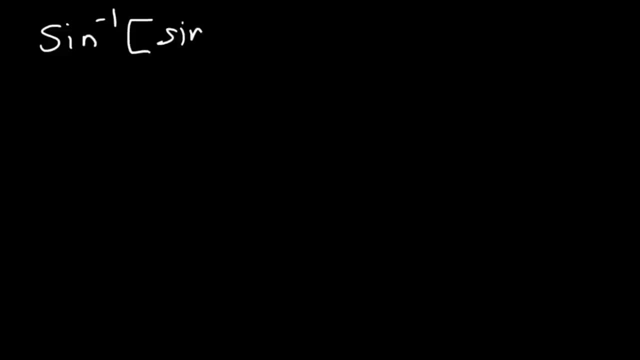 let's say, if we want to evaluate arc sine of sine of pi over 2, sine pi over 3.. What's the answer? For this particular example, it turns out that arc sine and sine will cancel giving us an answer of pi over 3.. 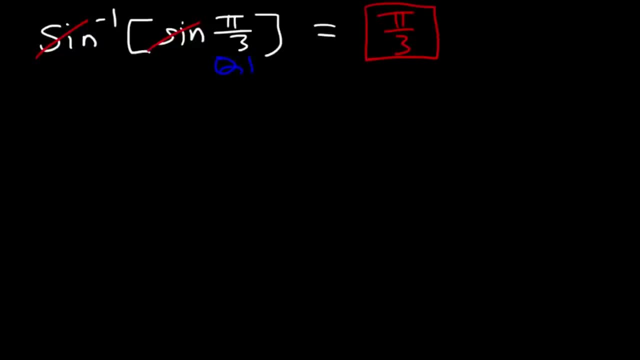 And we can do that because pi over 3 is in quadrant 1.. And arc sine exists in quadrant 1.. But let's take it one step at a time. So first let's evaluate sine pi over 3, or sine 60 degrees. 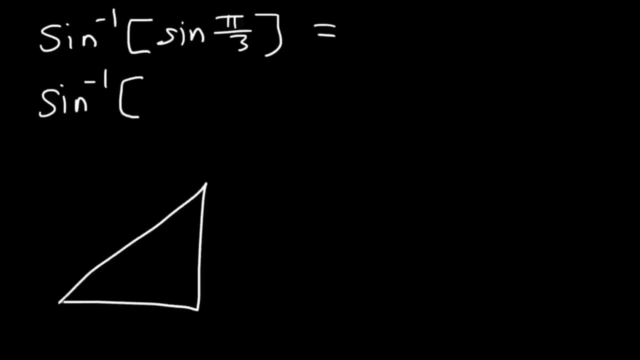 So, using a unit circle or using the 30-60-90 reference triangle, you know that sine of 60 is equal to the opposite side, which is square root 3, divided by the hypotenuse 2.. 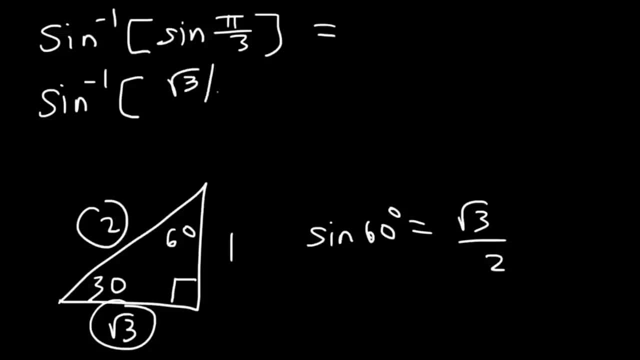 So sine 60, or sine pi over 3, is the square root of 3 over 2.. Now we need to evaluate arc sine. Arc sine exists in quadrants 1 and 4.. Now, because this is positive, 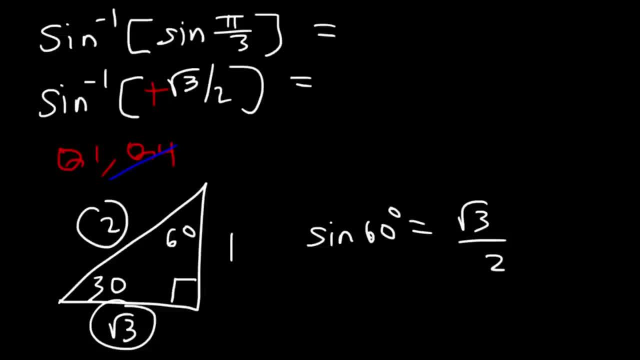 we don't want the answer in quadrant 4, because arc sine is negative in quadrant 4.. So therefore the angle has to be 60.. It's going to be pi over 3, because that is in quadrant 1,. 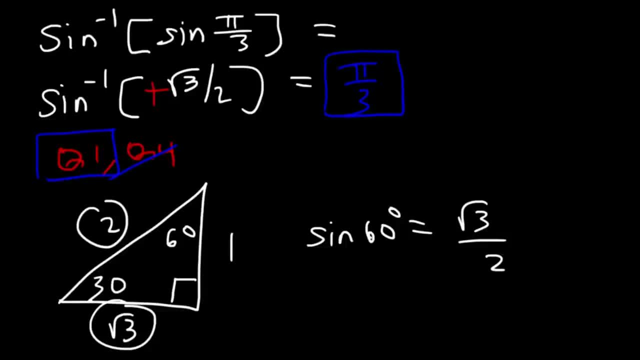 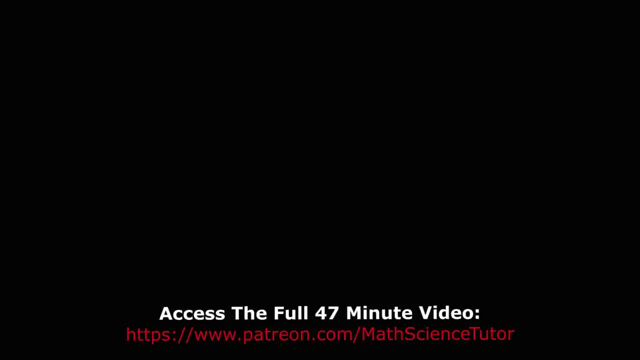 and arc sine exists there. So in this case, the final answer is simply pi over 3.. We were able to cancel these two. Thank you, Thank you.